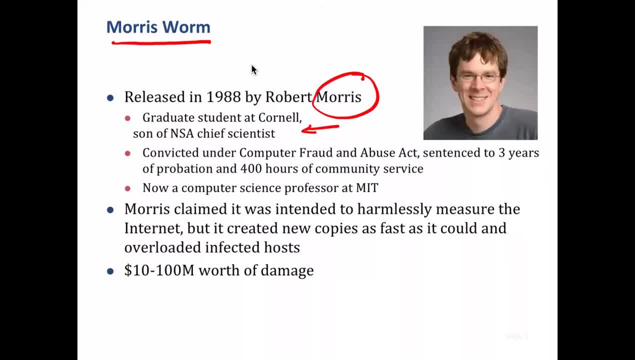 student at Cornell. Okay, This is a good school, one of the top, maybe in top five in US. And he was also son of NSA chief scientist. NSA- basically, you would have heard of it. It's an organization in US, right, It's a security agency. All right, He's a big guy, Chief scientist. 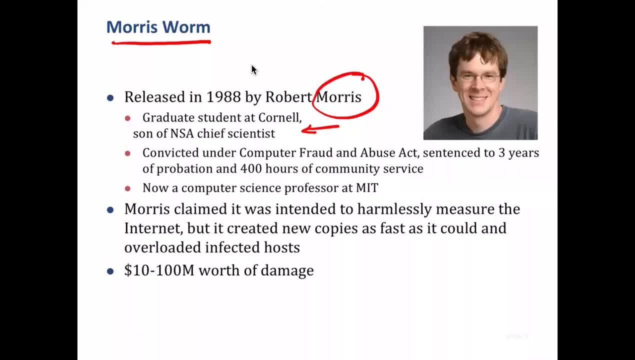 is a really big guy there, right So, and I'm sure he was very, very bright because he studied in Cornell And he was convicted under computer fraud and abuse act, sentence for three years and for 400 hours of community service. 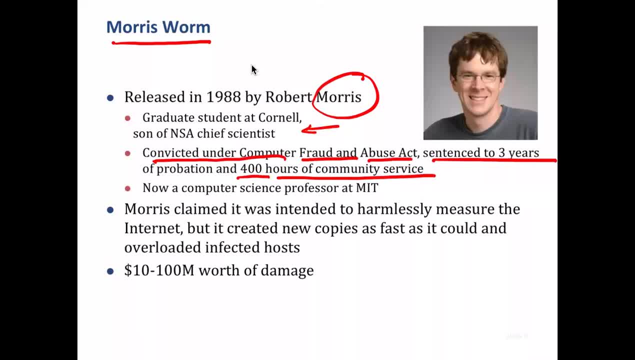 Okay, so, so he, he was very curious guy And then he created this, possibly for fun, you know a worm and injected into system and then it spread, Because see note that when we use the word worm versus virus, okay, when we use virus in general, maybe, maybe, 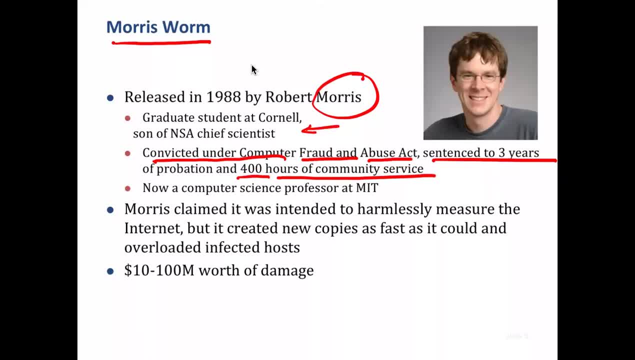 biological virus as well, Then a virus needs some carrier to carry it right. So, like the virus that we are facing nowadays, Coronavirus, if you sit in a room and don't go out, nothing will happen to you. Somebody has to come to you with the virus right, And then that carrier will infect you. 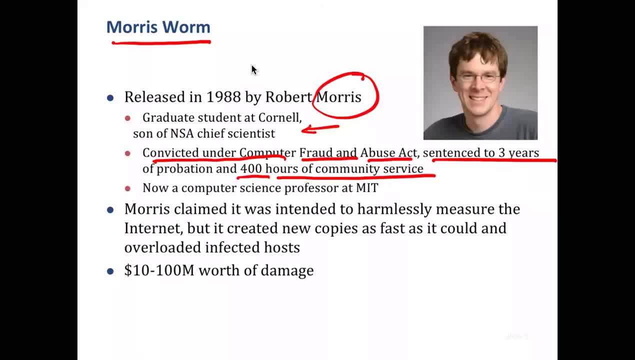 Same thing happens in computer virus. Computer virus come over something right. I mean, maybe maybe you have used your flash drive or flash stick is infected with virus and then you use it. then it transfers to your computer or it can come over email Within. 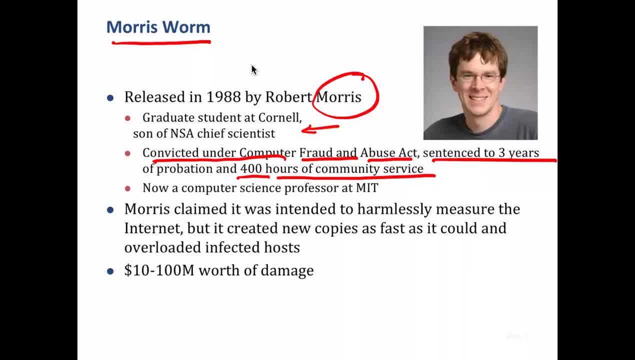 the worm has property that moves by itself, It replicates by itself And it does not require medium. So this elixir is already noihin virus, And warm is that worm can use mechanism for it's a movement and the application. 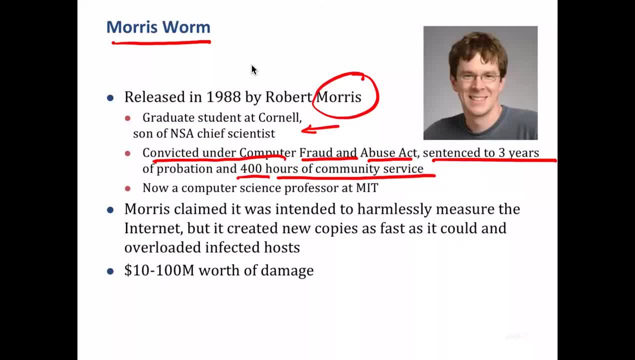 So basically a replication can happen, you know, without any medium. So he just created this for fun and wanted to test it, and then it's gone out and then spread all over the world. re 이럿 somm 메인 액테크리엔 전 병다의 복 abla 음 원 지�cha 용 bah. 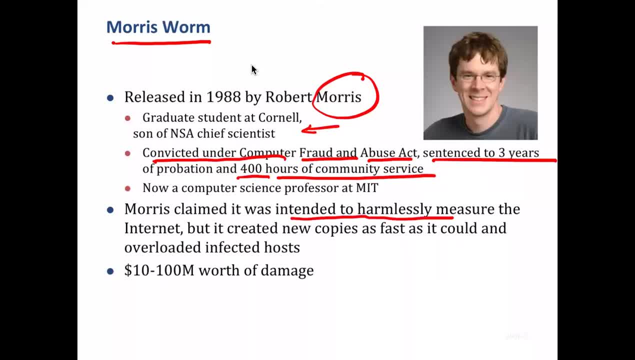 그리고 이것은 방식 격치가 있을 것이다 And he claimed that he intented to do. basically, its intention was good, not causing harm to anybody, but it created new copies as fast as it could and overrated the infected host and amount of damage was 10 to 100 million. 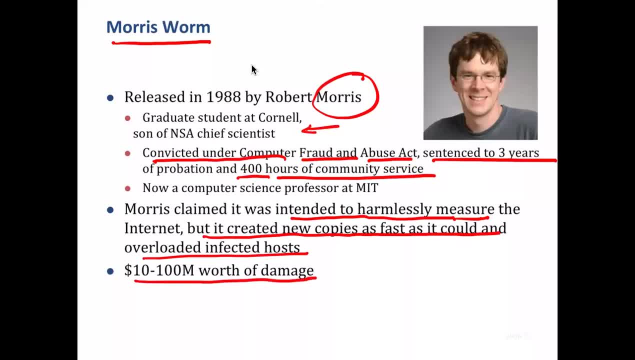 okay, obviously, when your money, for example, you are running a company and virus infects your company, a worm infects your whole organization, it you have to shut it down or so you have a losses right and for you who has losses, it is a criminal activity. you know- and you may not think that you know- some nice person who's studying in. 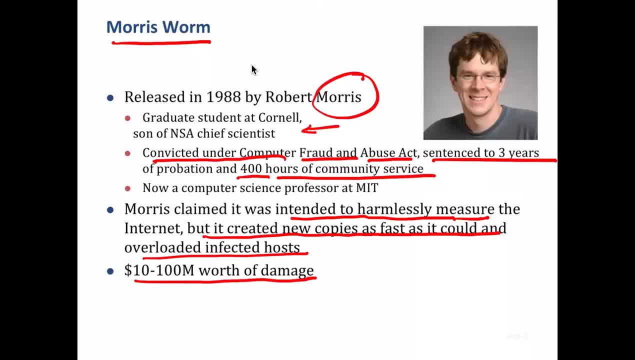 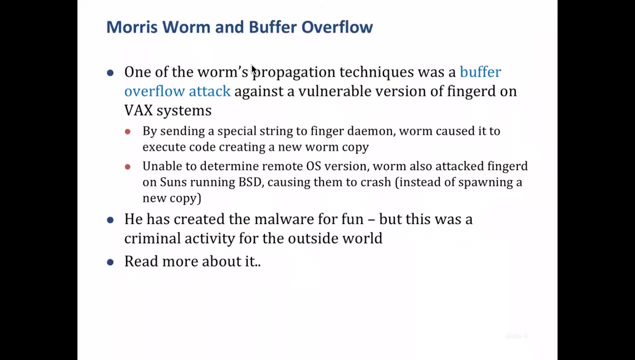 Cornell has done this right. so what so? so that's the reason he was convicted. but now he is a professor at MIT. possibly you can look at his LinkedIn profile and so on. okay, and why we are discussing this is because the worm's propagation technique was using buffer or 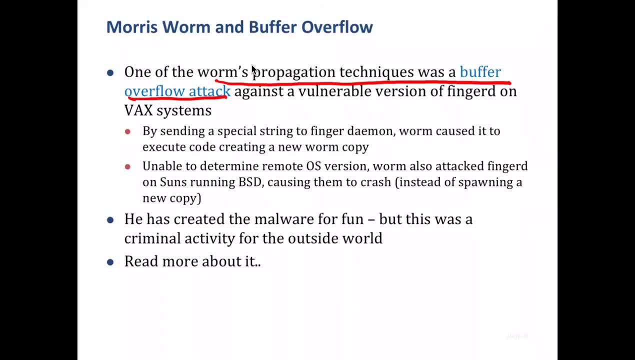 flow attack. okay, all right. so basically, I mean, we are not going to get into how what he has done and so on, because you need to understand wet system and then we'll have to see what some some feature that he has used, some some function which is fingered function which is fingered function. 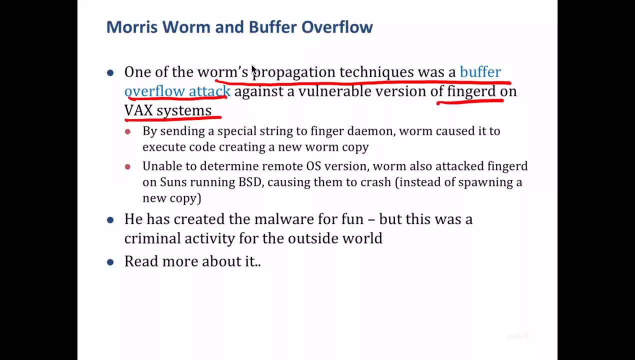 and you know so. it is basically by sending a special string to demon, finger demon and worm, cause it to execute code, creating new worm copy. all right, so I will request you to please read more about it. okay, so when you are developing a malware, even for fun it can- it can be dangerous, right. okay, so when you are trying to 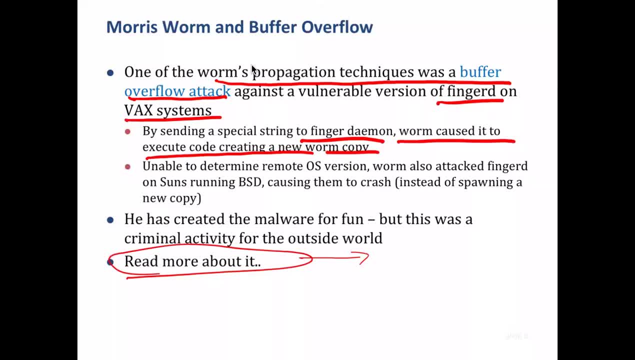 learn hacking, which is ethical hacking, and you had by mistake some somebody's computer- even my computer, for example, or or any computer in institute, then it's a criminal activity, right? so if you are doing criminal activity then you can punish. so best way if you really want to try, is that take approval that I want to. 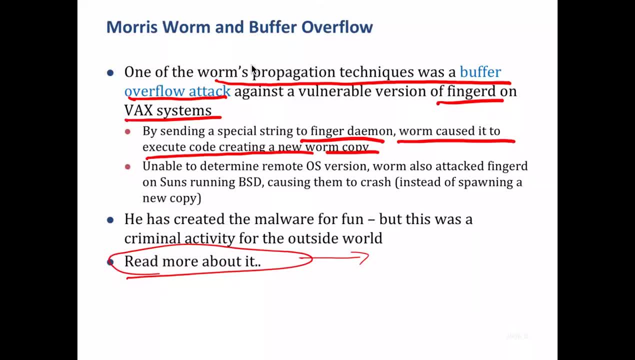 hike your machine, could you please allow? so? there's the best way, right, okay, okay, and that, and you can get paid for that. okay, many companies pay external agency to get into their systems. okay, find holes in the whole security thing and then by once they know what are the holes, then they can plug those holes. right, there's a very simple. 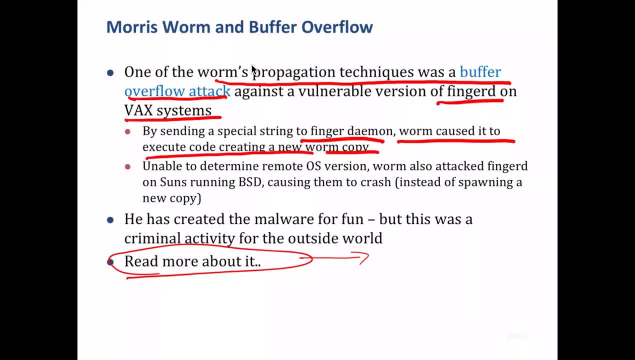 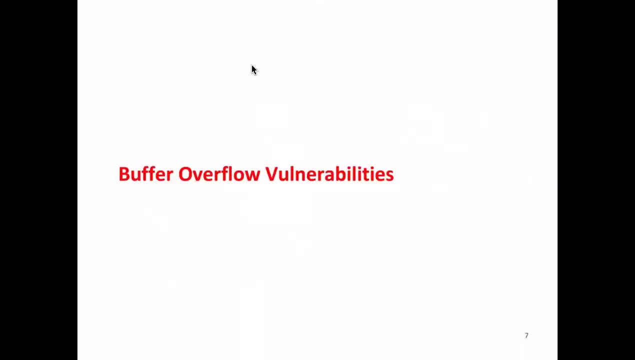 way of, well, less expensive way of finding out the holes or vulnerabilities, right so? or vulnerabilities, okay. so with this let's start today's presentation. okay, why are we studying this? because this is still the most used vulnerability. all the most of the OS and new chipsets have taken care of this, but 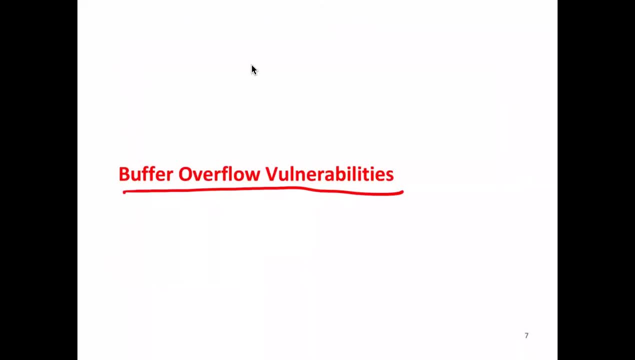 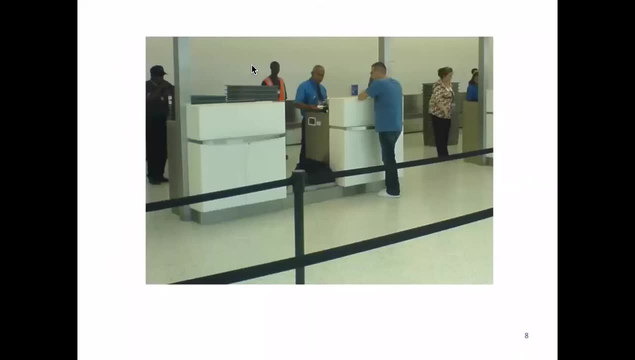 still, you'll find lot of old servers running that have still these holes- okay, these kind of vulnerabilities- that have still these holes. okay, this kind of vulnerabilities. okay, this kind of vulnerabilities, okay. so this is the diagram where you are, this scenario where you are in airport. okay, what do you do? you just give your copy of ticket. if you have in many countries, like 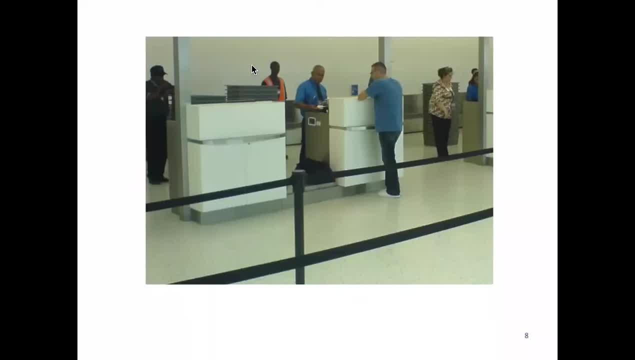 us. you just need to give your passport or some identity card, okay, and then person based on that person will find out more about you and then issue a boarding pass. okay, so this is the process. okay, so, but in order to do that, you will have to fill up a form, right? 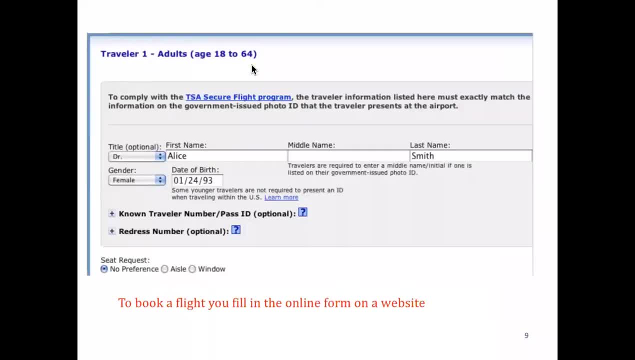 make a reservation. okay, so you have filled up the form. this is basically form in us okay, base any application and it could be through any website, but i internally, you know the interface could be slightly different. or, finally, same data will go to back-end computers. right, and this is the way it goes. this is the form, okay, wherein there are fields, like you know, name. 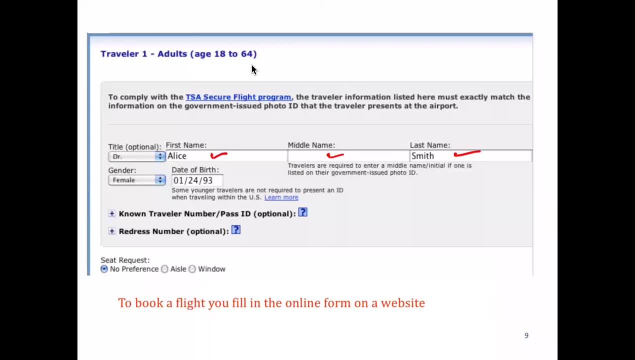 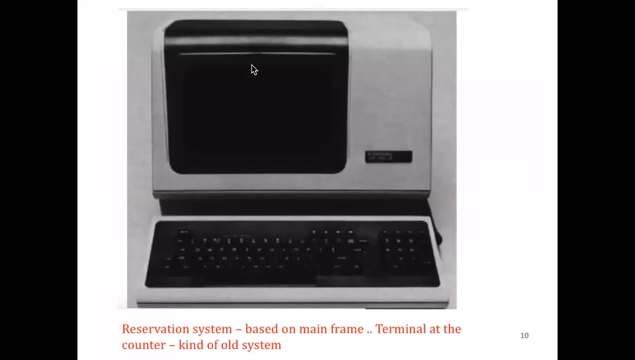 first name, middle name, last name, okay, uh, date of birth, etc. okay, gender, uh, and all that right, okay. so you'll have to fill up this form and now this will give you some information and then, based on that back-end, will do some reservations and then when you go to airport, it will look on the terminal, something like you know, uh, something like this: 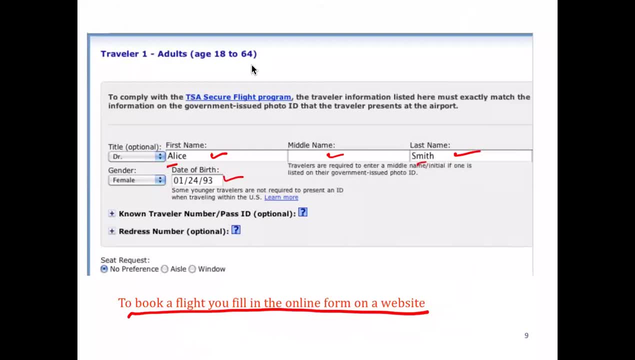 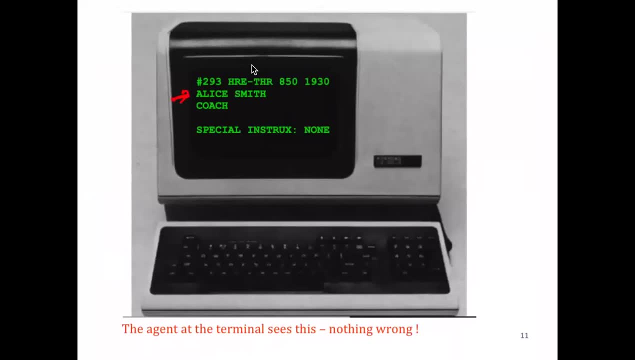 okay, so she has filled in this her name as alice smith and so on. right, so it will appear like this: that are: this is the name and this is a class coach class we, which we call here as economic class. okay, and any special instruction name. so this will appear on the terminal of: 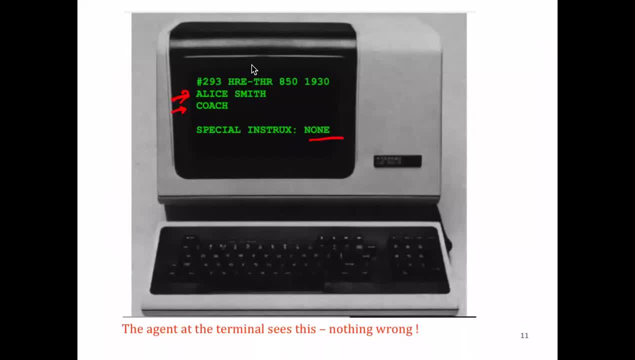 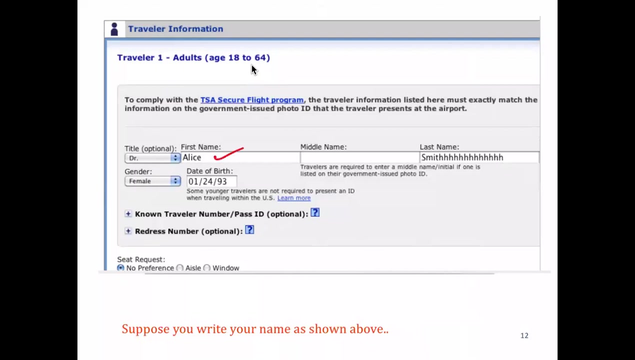 the officer or or the person who is doing check-in. all right is. is anything wrong? do you see anything wrong in this one? nothing, okay, it's fine. okay now if she does the following: okay, first name, she writes. as it is last name, she write smith. then extended this hh, set a number of. 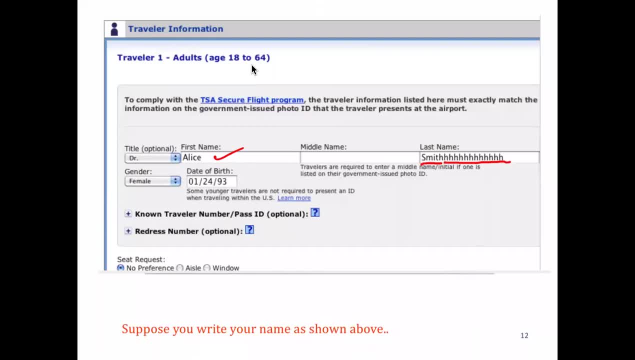 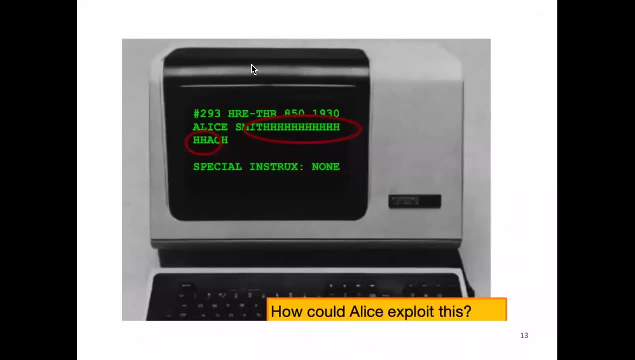 hs right now, this will system will accept it, because name could be anything. okay, nobody stops you from putting so many hs again in your surname, right? and then it will appear something like this: do you see any problem here? any problem: class is changed. yeah, class is very good, class has changed. now you as a hacker, you. 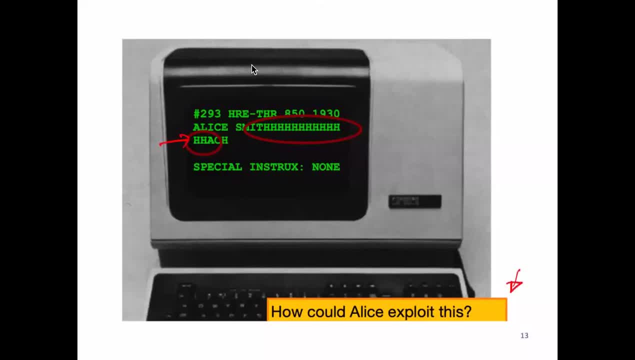 want to take advantage of this vulnerability, and this may not be a crime. actually, you are doing best from your side. and then, if system is bad, what can you do? okay, what can you do now? now, instead of hhs, you put something so that this becomes, you know, economic class, to say, coach class. 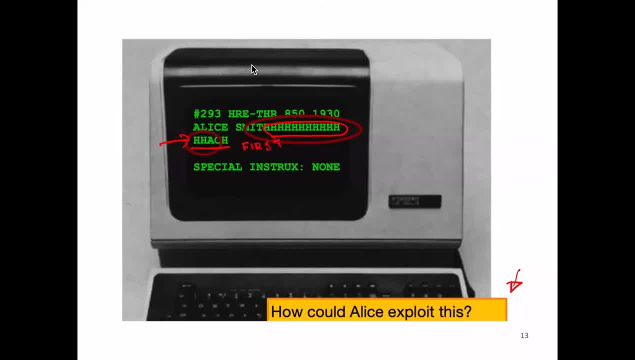 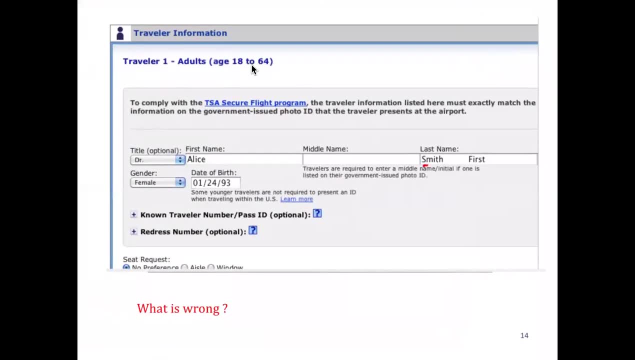 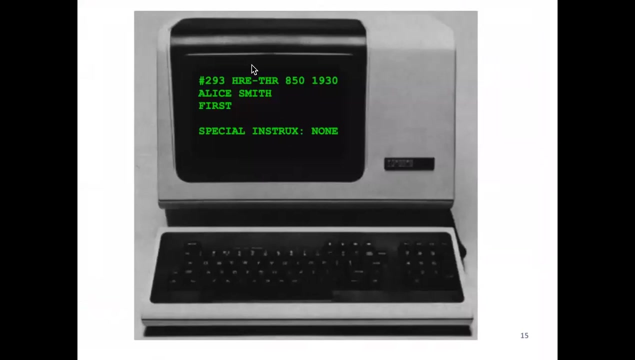 to say first class or something like this, or business class or something like that. okay, so now, if she writes something like this, you have the ability. what can you do? that is when you have the ability to go right by now, want to bring her a string. I don't know what I want to do. come here. 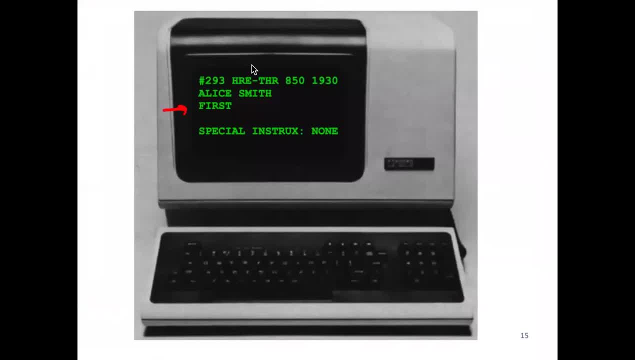 I will name the CSS, because if I want, I have to go first right, ref, congratulations, correct, and then she writes. she writes something like this: this one right, and then you write the second one for clamps and certain number of spaces or blanks, and then right first. okay, then this way it will come something like this here: know that this is an example. program logic could be have more checks, but this was actually a vulnerability in the lacks most. this is fine, look, and then, if this is an example, program rights as well, but I hope she knows not. so that isивает has the ability to be more necessary, but this was actually a vulnerability in the packs of. so there is nothing. we didn't know. that really, all right. 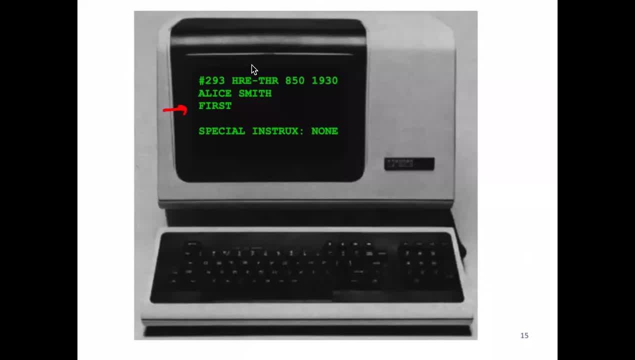 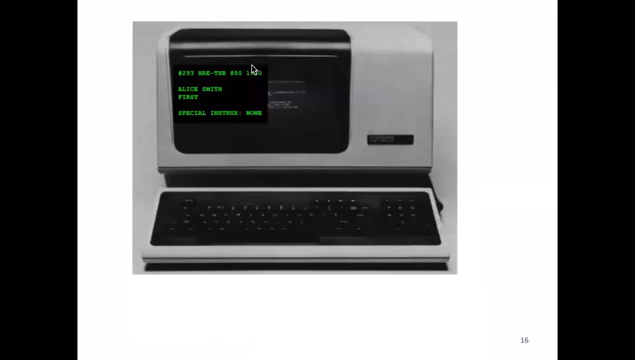 class. So now, what ticketing agent will do? Will give her a boarding pass with first class seats. So now, where is the problem? Problem is here: By inserting padding characters or spaces and exploiting the lack of boundaries between the lines, Alice now appears to be. 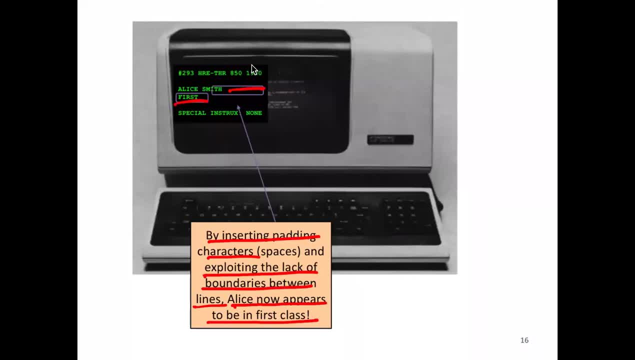 in the first class. It is fine, but Alice has to be smart enough to find out how many spaces to put, Otherwise the first will not appear in the right place. So attacker can exploit lack of boundaries to control areas in memory which they are not supposed to. 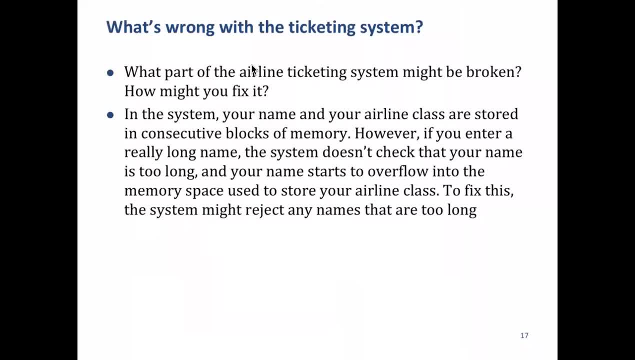 do So. now we can see how what is wrong with the ticketing system. So here the problem is that your name and your airline's class class are stored in consecutive block of memory, And if you enter a really long name, like Smith, H, H, H, H or whatever, the system does not check. 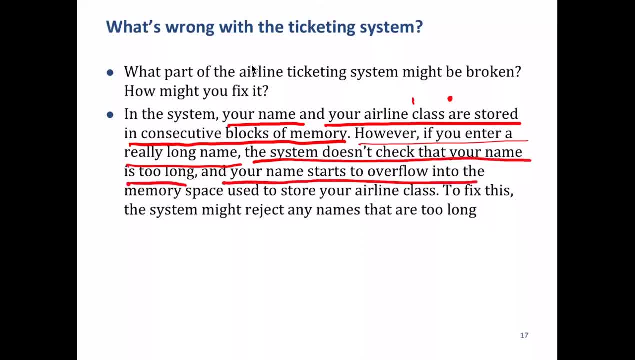 That your name is too long and your name is such to overflow into memory space used to store the airline class. You can, of course, fix this, you know. but when you are right doing the, you know whoever has done the programming might not have thought about you know, anybody. 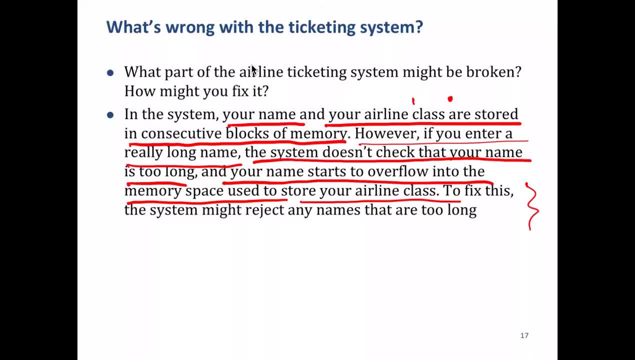 can exploit it If the programmer think about these problems right in the beginning, because security is never in the mind of programmers. They never think. I mean I have not seen in my career anybody thinks about security. They think always about efficiency. Okay, and 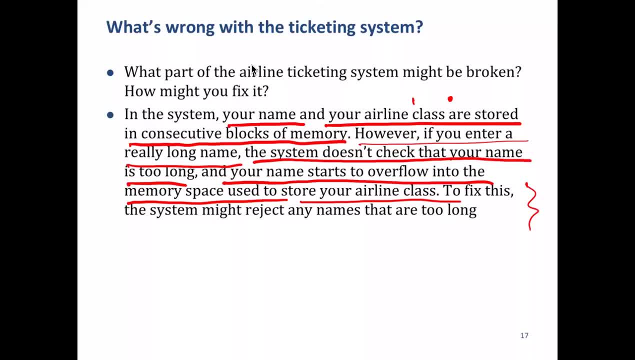 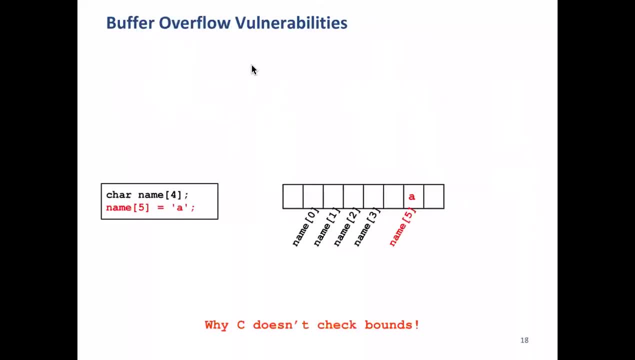 other factors, But if the security thing is kept in mind, then this problem can be avoided. right, All right. So now look at your favorite programming language, C. Now, here you define an array, character array. Name is character array with size four, Okay, four bytes Okay. And now you store into fifth. 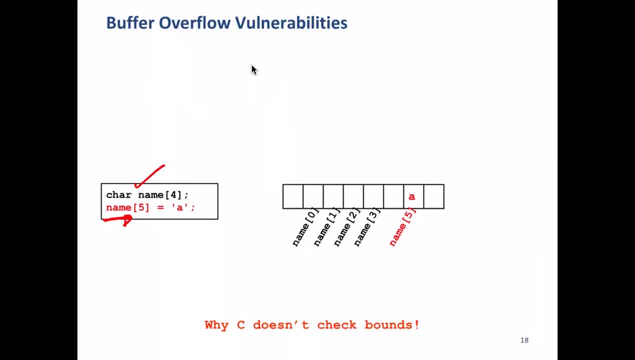 location: Okay, Name five, some some character: A: Okay, This thing you are, When you know this thing goes to. Basically, it is created in stack. Okay, because this will be created. This is all temporary thing is a variable, Right. 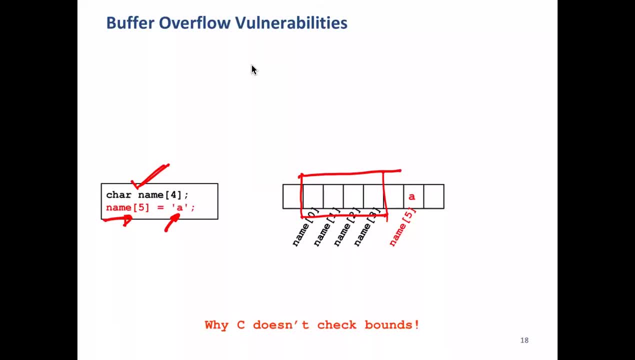 Okay, It will be created in a stack. Okay, run time stack. Okay, that we have seen. I mean, this is run time or Memory image, and you have. you have basically text, whatever you have seen in the last class. right, then you have heap and then you have stack. I am just for simplicity, let us assume that 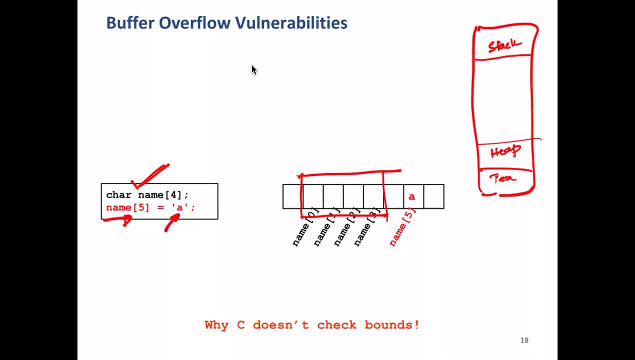 this. So in a stack, you will, you know, this variable will be stored. ok, this, and now, of course, there will be memory location adjacent to that. ok, So now A will be written there here, in this location, right, because 0, 1, 2, 3, and then you are using fifth element of. 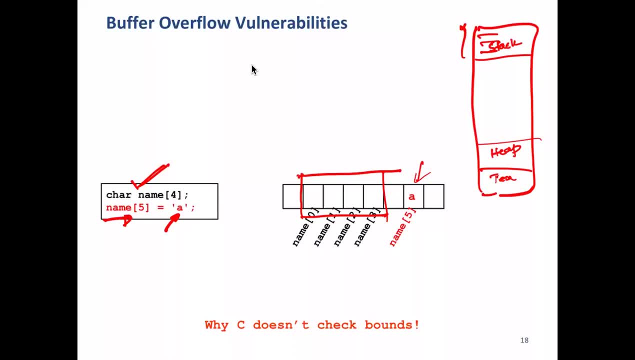 this array, So it will come here. if you use fourth element, it will. should would have come here, right. So now the question is that C in general does not check bounds. Why? why is that? See, this problem would not exist in safe python, So C is called memory. 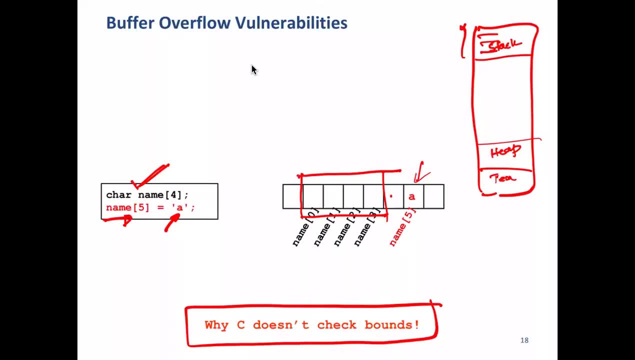 unsafe language. Now, the designer of C gave the power at the hands of programmers. They they assume that all programmers are bright, intelligent and will not make mistakes. this is a power. okay, it gave very less power to compiler, etc. right, so so these checks are not done. 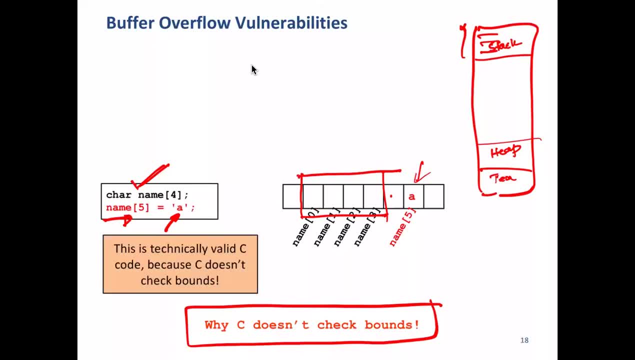 okay, let's move ahead. so this code is technically valid but doesn't check, bounce right and and hence there is a problem. so, largely because she has no concept of array length, it just see this as sequence of bytes. now, if you allow an attacker to start writing at a location and don't define where they, 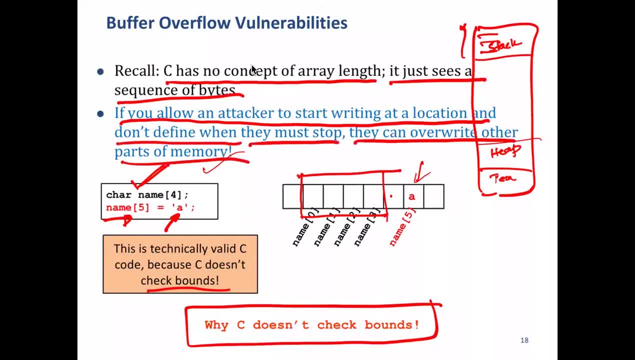 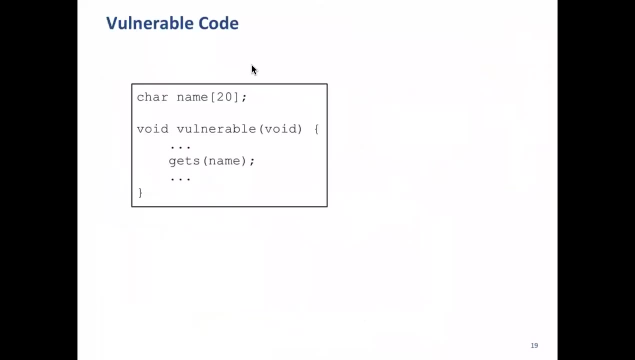 must stop. they can overwrite into other parts of the memory. so there is a learning. so attacker can use- you know location which access location and can write on location which they are not supposed to. So let us look at the example and become clear. So this is a code, the C code, and we call it one. 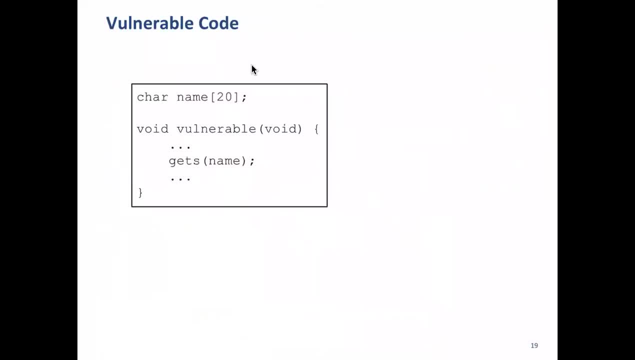 rebel code. yeah, just a minute. all right, This is a function and before that, before this function is called. So you have array called name with length is 20, all right, and then you get your in that function. you run this, gets name It. 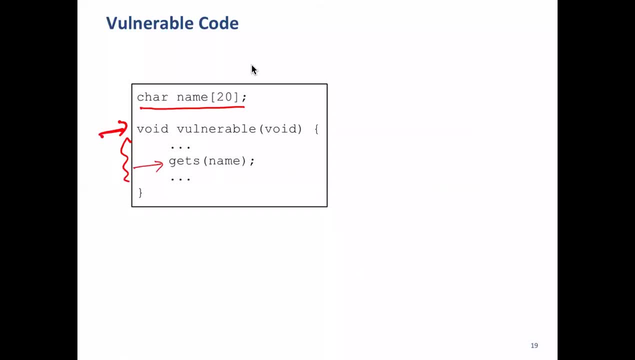 remember what is gets gets what. what will do anyone input string? yeah, input string. right, you can do it from keyboard. all right, So now let us see what will happen. So gets function will write bytes until input contains new line character. okay, not when the end of 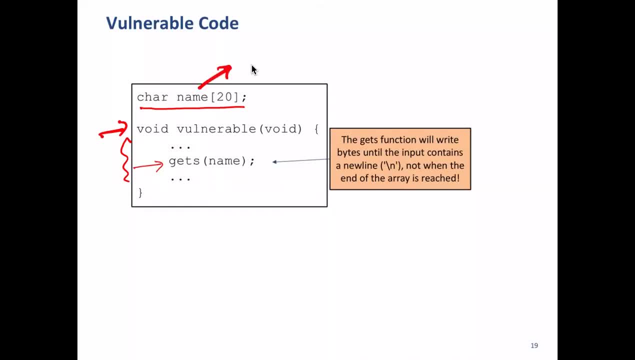 array is reaching. So essentially, if you are writing in name array its of size 20, you define this of size 20 and you get a string called name and then string. you know this function will check only this character, new line character. till that time it will assume that this there is a string. 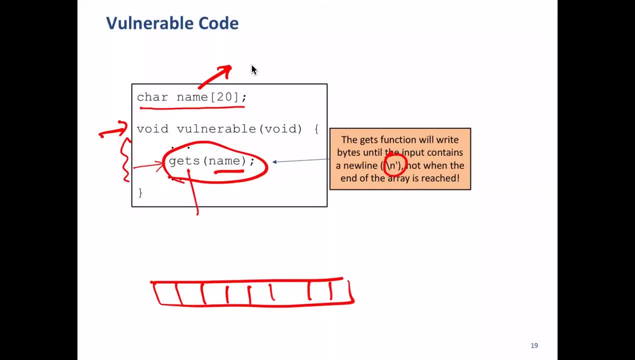 okay, So string one is So. string one is So actually starting in this function. we here we need to write its elder. there is a little link for g ref number here. what is it? just two frame, do not be filled. this it. 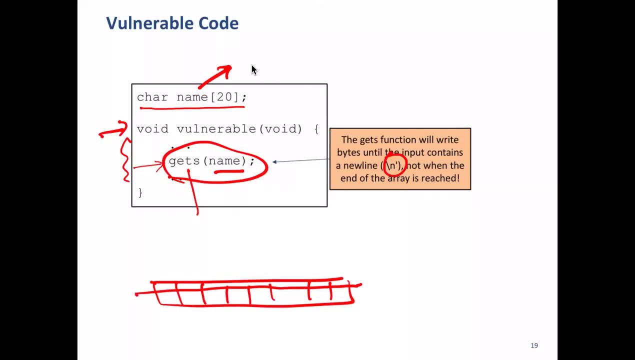 comes so severe, we will start filling this. it does not bother about whether it is 25 bytes or 30 bytes, until you it gets back a new line character. this will continue to write right. So all this location can be written if name has more than 20 bytes um. 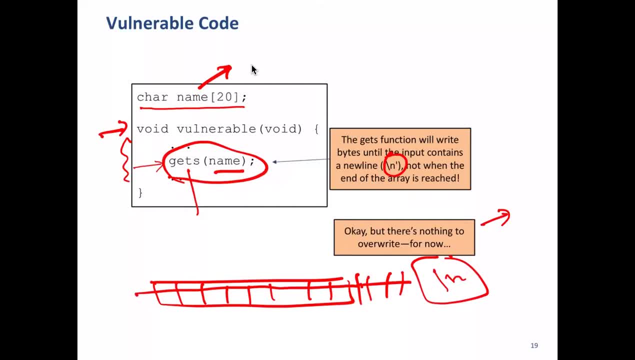 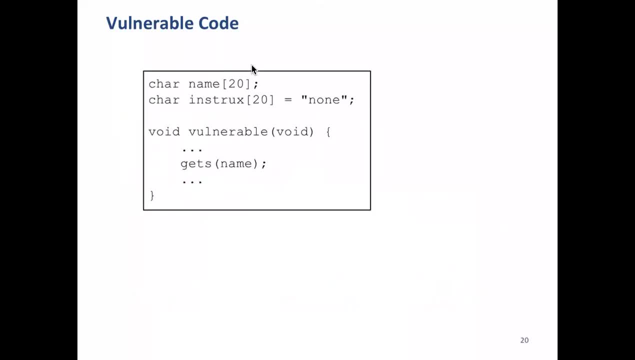 this is fine because there is. you know it is. even if you write something here and there may not be anything useful, it is ok. Now let us look at this example. ok, So this is the same. there is a name is array of size 20 and there is another array which call instructs. 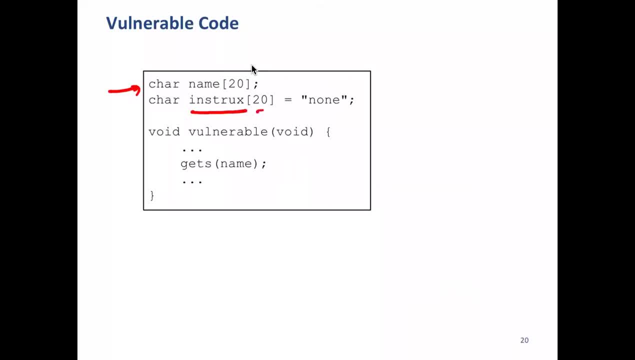 instructions essentially of size 20, and then we assign this as value none. It means there is instruction which, if this value of may program logic is something like this: if this value of this is none, then do nothing. ok, Alright, now you run. this gets name, So what? 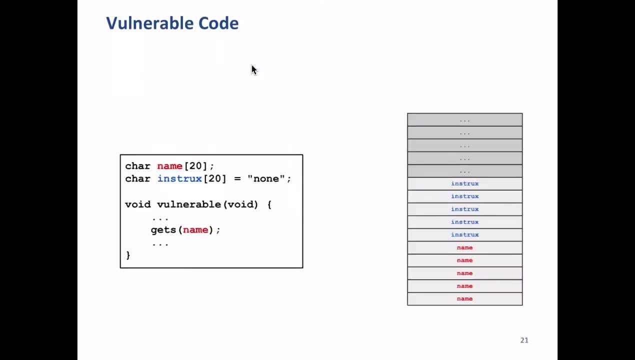 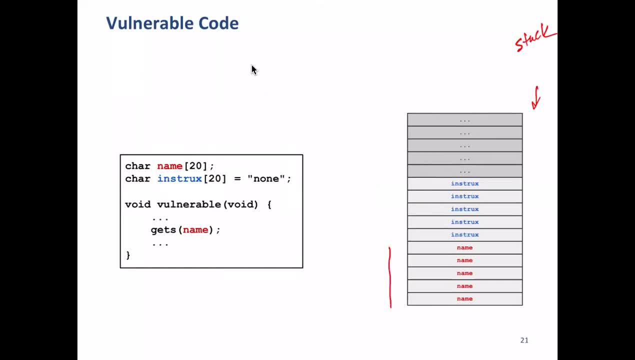 So it is something like this: this is your stack. Okay, so a stack. these will be reserved. Okay, so a stack. these will be reserved for you: the 20 bytes, and this is one word of four bytes. it will start from here, it will go up to this point: one, two, three, four. 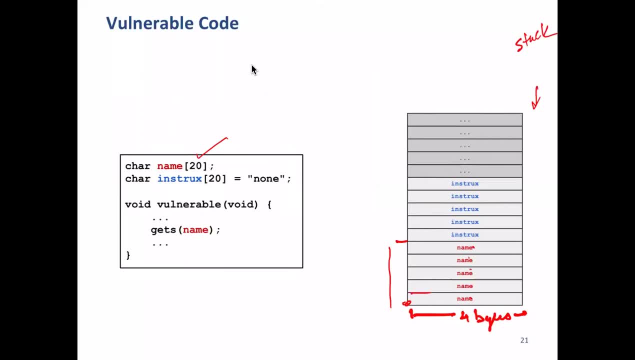 five, right? So 20 bytes where each word is a four bytes. okay, and then it will desire. okay, it will reserve space for 20 bytes for instruction. So this is the compartir function: space for 20 bytes. So, right at this point in time, no values has been assigned, right. 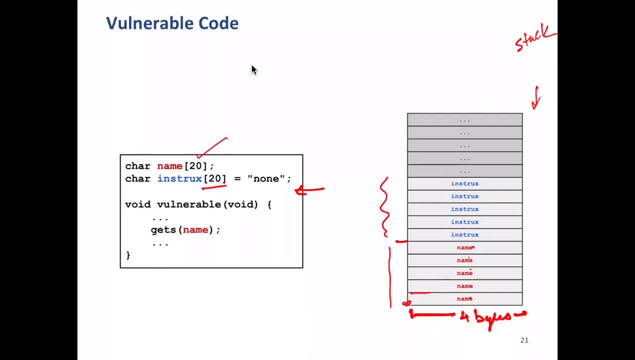 So you just set this, space is created. All right, Now control comes here and this function call or the sorry, this, this uh statement is run. Okay, So it's a gets name. Okay, Now writing starts from here. it goes upwards And if a name that you're entering to keyboard. 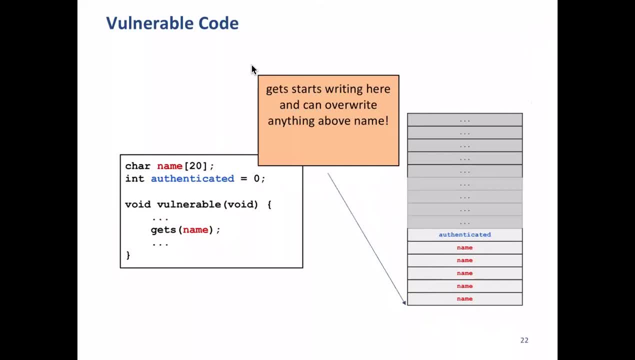 is very long and can overwrite here. Okay, All right. So now you, we can see that, uh, you know this, this can be overrated and this can be exploited. Okay, By uh, when program ransom next, or sorry, you let. me put it here. for example, I have this script now which is going to wait for five minutes itself. So, starting from refresh the thing that your type- Uh, What that script expressing Vocal starting from response can be an overwriter. that's broken down. Let me put you up here. 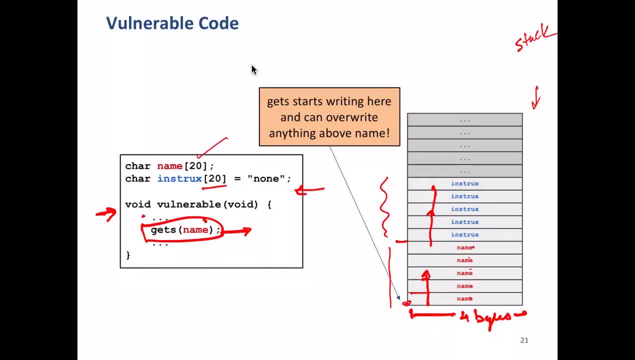 in the, you know, further execution of the program. after this and when the program logic checks: if the value is none, then do something. it finds something else, All right. so this is another example: name array of 20.. So in the stack these four words will be: 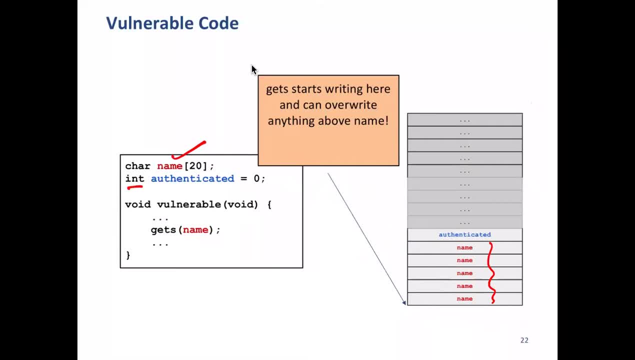 reserved for name. and then there is an integer which you are defining is authenticated, this authenticated, So it will be assigned value 0 and you get you read a string name. okay, Now you can make this instead of 0 as 1 by having something here: 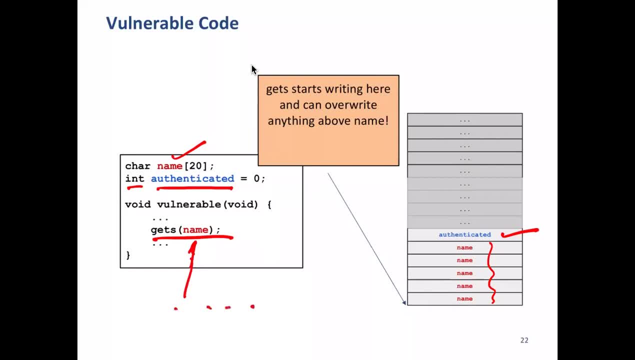 in the name when you write, when you, when you, when you equi type. okay, Similarly, you know. so, basically, instead of 0, if you, you can make it 1, because you know, with, with 20 bytes of name, whatever it could be, say 20 bytes, let's say the 1 up to 20.. 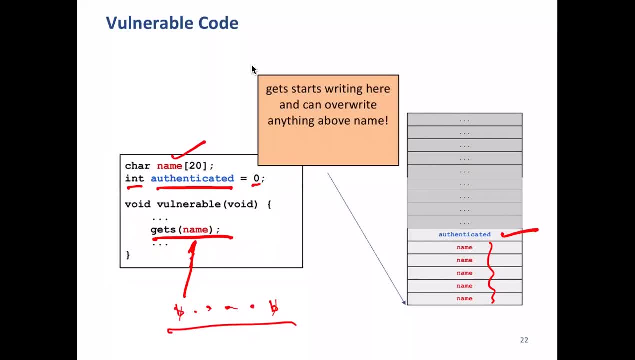 So these will be filled with some characters, say b, for example b or whatever, or maybe 2 times b or whatever. you have to calculate right how much what you have to do. p, b, b, b. each character cell, racism, is 1 byte, So 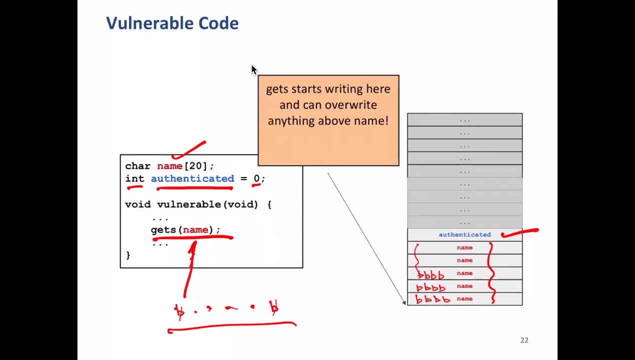 so you do it okay. okay, all right, and here you put 1.. So string could be: you know. now note that it's a little endian, so you'll have to find out the sequence. what is the right sequence? it could be 1 b, b, b, b. 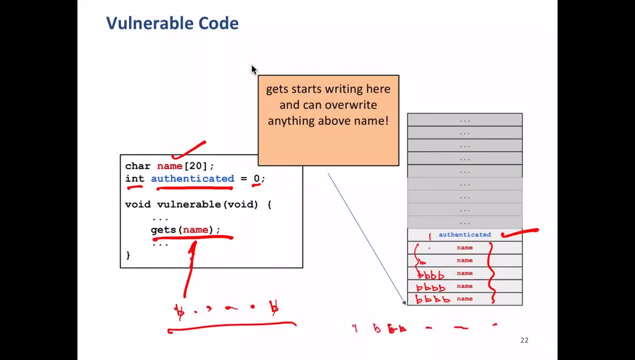 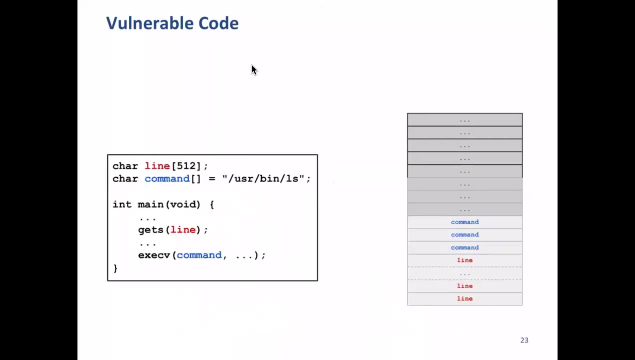 something like this: and then this will becomes 1: okay, So now something that is not authenticated becomes authenticated. So this is. let's look at another one: the ability. okay, just a minute, sorry, okay, So let's look at another one. 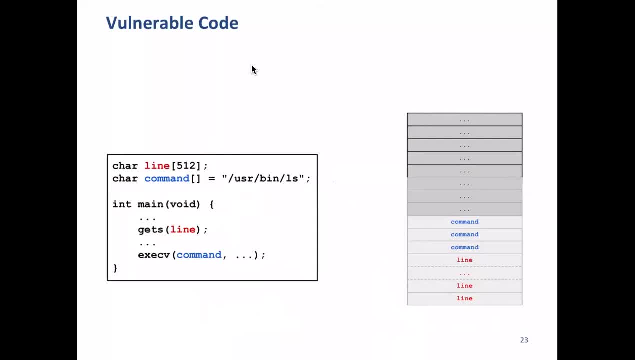 So let's look at another one. Okay, here we have character array of size 512.. Okay, so in a stack, this is, this space is reserved. and then there is a character string, which we define as, which is named as command, which is of 12 bytes, the one here: 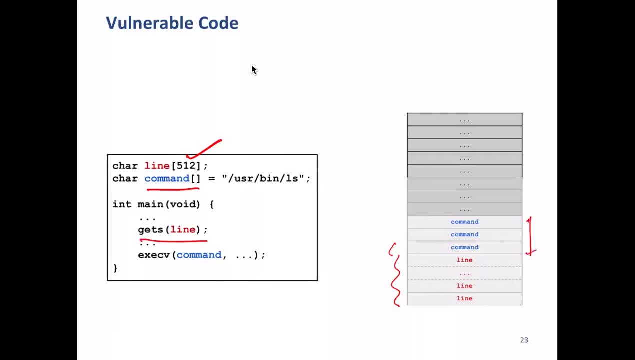 Okay, all right. when you get slime, you can do one thing is that you intelligently put whatever command you want to execute here, which is malicious command, which is it's not supposed to, okay, Okay, and then you have a exec cv command. Now note that all these things is in a machine instructions. the program is running this, so 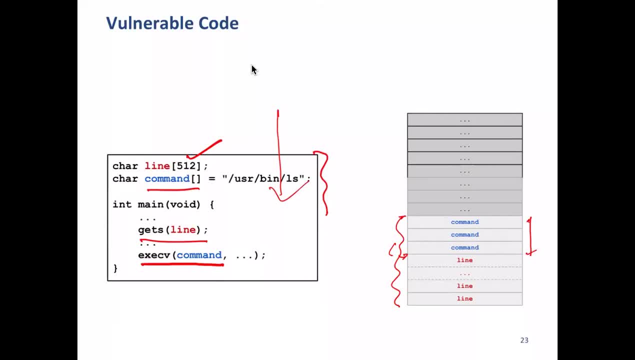 a hacker will not know what. all this is right. So it somehow assumes that it could be command there. okay, and then- because this thing may not, all these things are not known- all he gets is a portion to type something, and if it types here some command, the command is not known. So this is the command. 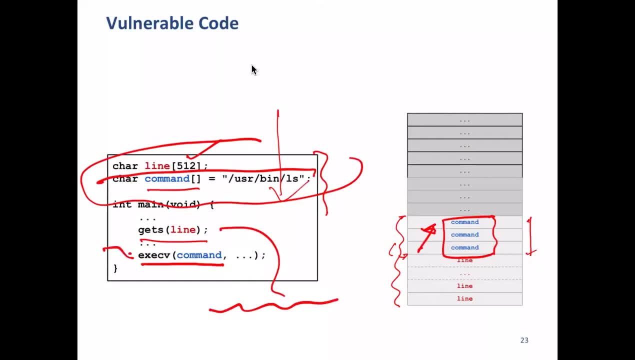 It gives you just as it said. the command will come here and then in the program if there exccv- I mean you know what CXCV means. right, because we have learned this in part of process. right, So this command will start running. it will. 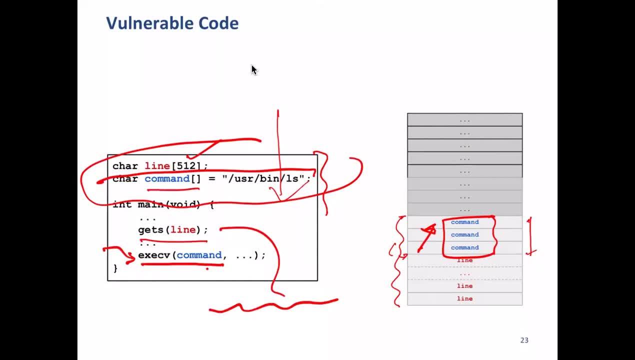 this? essentially it will change the code of the process it created and you know the process code will change and then this command will starts running. Then this command will starts running as part of the main process. we fork it, then we run exe, cv, right, then then fork process starts running that new code. similarly, 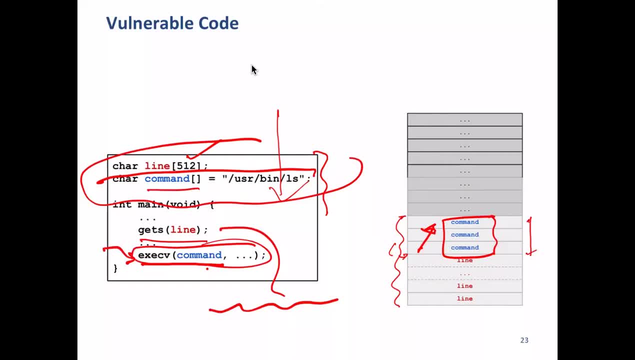 here. you assume that it's not forking is not happening. execs, we directly are running, so the code of the running process becomes a new code, which is that of a command. okay, all right. okay, what is it happening here? what is this thing? what is this? 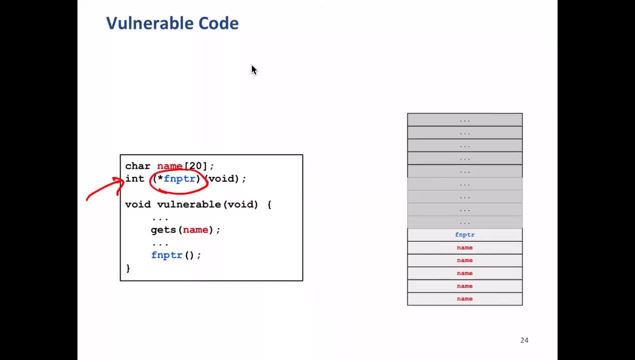 anyone. function pointer is a function pointer, right? we studied this in in uh os course, right? for others who have not studied function pointer, please study uh function pointer. not many of us use this. you know this. what do you call that feature of c? but this is a very interesting way of using it, right? 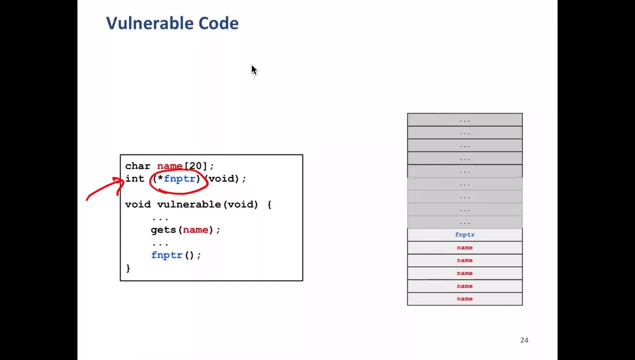 okay, so this is a function pointer, essentially a pointer to a function. okay, so i mean in other ways to when you call a function, actually implicitly compiler does the same thing, but here explicitly you define function pointer. okay, so what? what's happening here then? uh, when in the stack first we have 20 bytes for name. 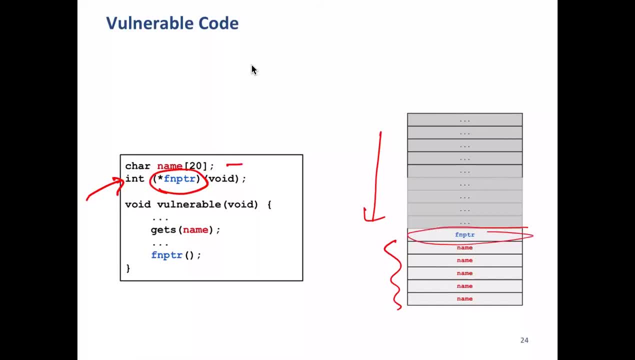 and then four bytes for function pointer. now even function pointer command comes and this function- then actually control- goes to somewhere right where this function points. so this is a pointer to a function and function may be somewhere here. so if we start pointing to starting instruction and then that can get executed, okay, but this has to be written. 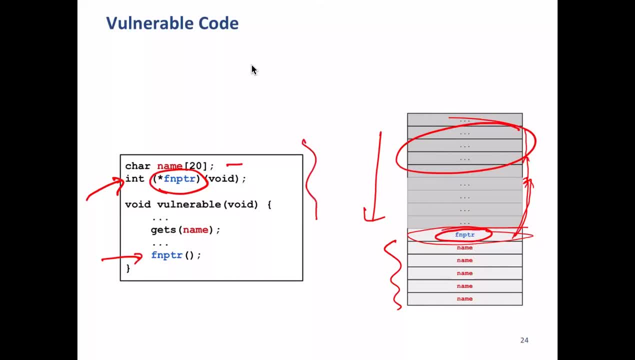 appropriately then, because all these things again is not seen by hacker. okay, hey, because there's a machine instruction. now there is also possibility in, uh, you know when source code is known, because you know, uh, for example, linux and many other man, for a lot of application source code is known and this vulnerability is visible. 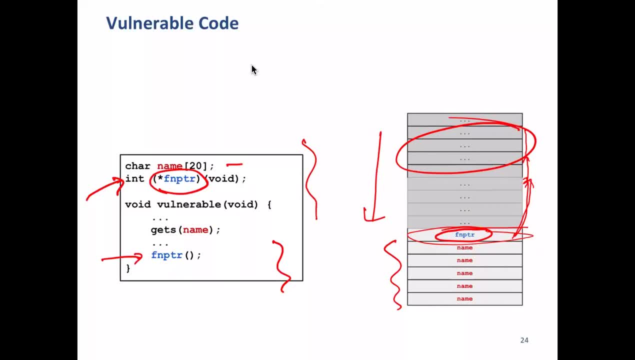 then hacker will know that, look, there is a vulnerability and this can be exploited. but in general, commercial software, like you know, whatever microsoft and google and many others develop, source code is not known. so now hacker has to, you know, think, try but assume, attempt and then try to find out vulnerabilities. 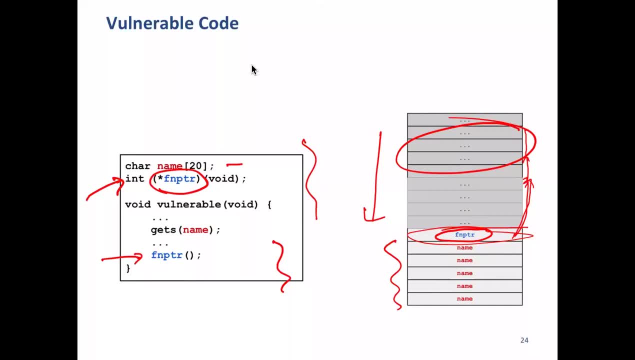 okay, any question up to this point. note that we are talking only about stack, which is in the runtime image. right, when the process we when program we execute, it creates a stack during execution of that program, that becomes process. okay, so we are talking just about a single frame in the stack. okay, so this all is a stack. we are not talking about heap and so on. 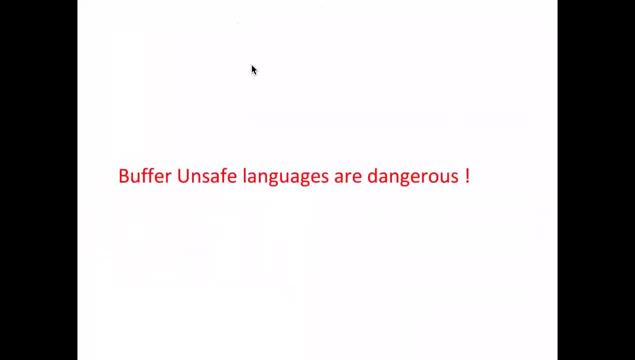 okay, all right. so buffer: unsafe languages are dangerous, which is c and c plus plus. they are very powerful and that's the reason they are used heavily in, you know, any system design and also it has been used heavily in application side, but python etc. are now changing it because of different reasons. 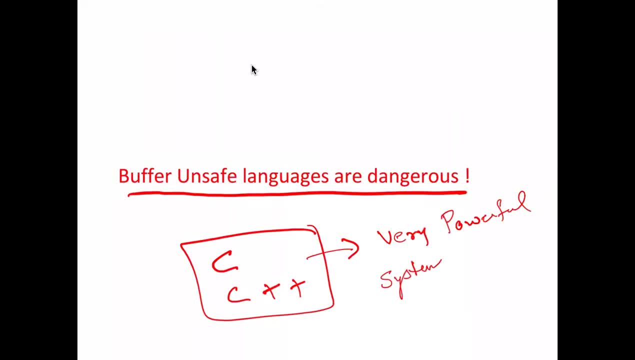 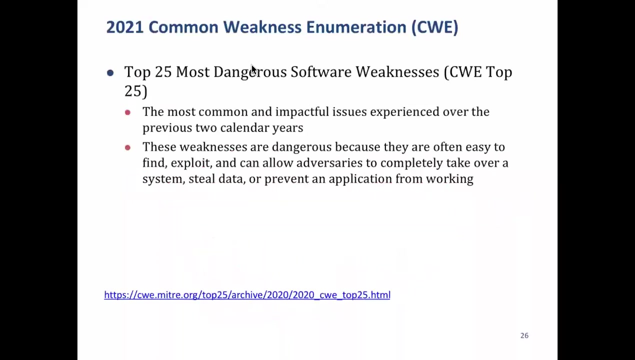 c is also very efficient, does not require too much of space in comparison to many other languages. but now space is not really the constraint. earlier, when the space was, you know, when we had just 64k of memory, ram memory- then all these things were very important. but not anymore. all right. 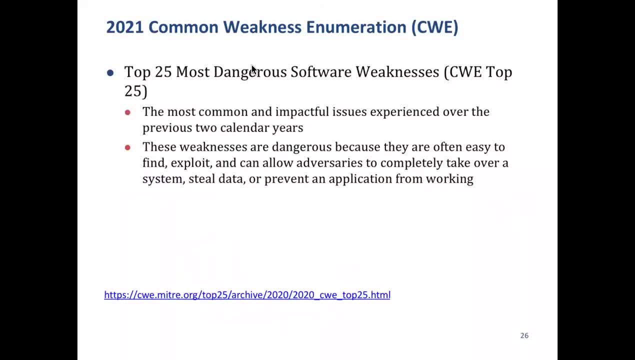 now let's spend few minutes to look at what are the common weaknesses that has been found by a group called cwe. you can go to this. this is a forum that that finds out weaknesses, right, so you can go to this link and find out what are top most weaknesses in this year. okay, all right. 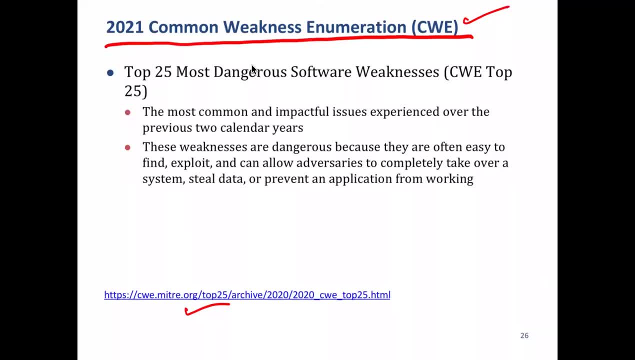 here they have. they list every uh all weaknesses right, and i have subscribed to their uh email, say, whenever they find a new weakness, not this one, but there's some other agency, government agency, us and in us and they keep sending me email. okay, so now this list has top 25 most dangerous software weaknesses. 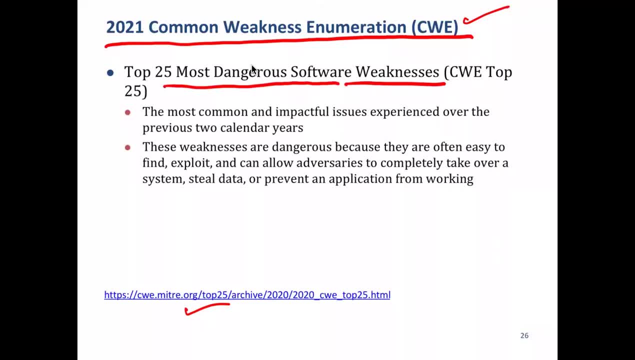 okay, okay, most common impactful issues experienced over previous two calendar years. so these weaknesses are dangerous because they are easy to find, exploit and can allow adversities to complete takeover system, steal data and prevent the application from working. okay, let's look at what are these. you double click on this. you will get that one, the one that's shown here. 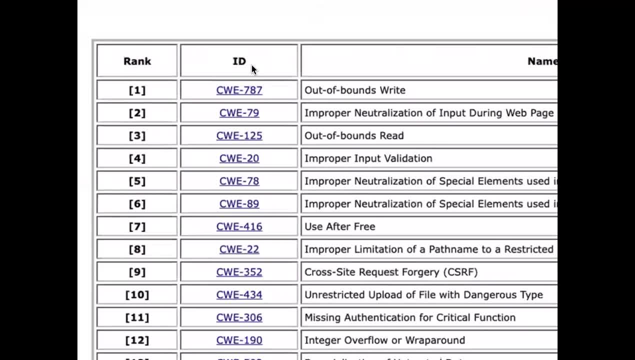 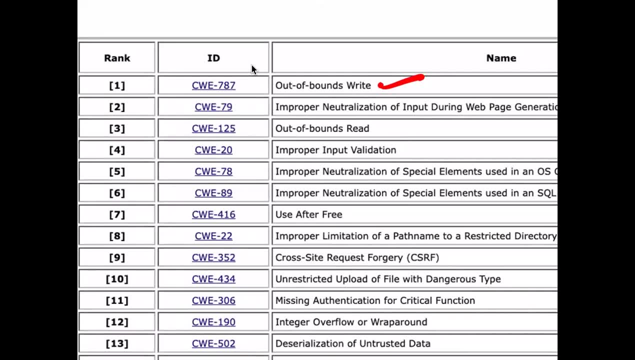 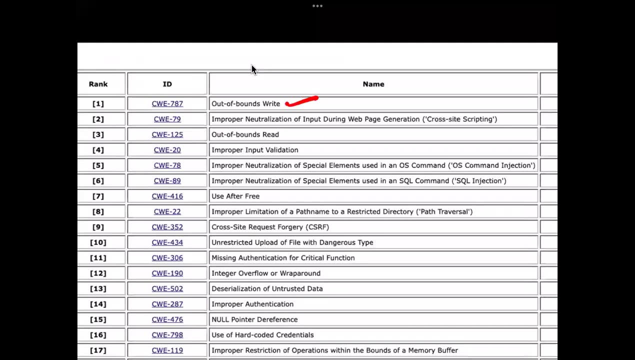 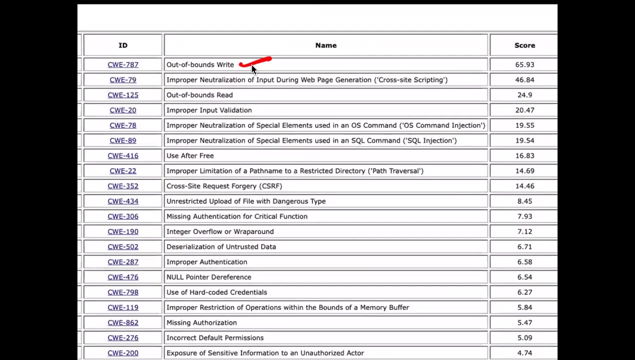 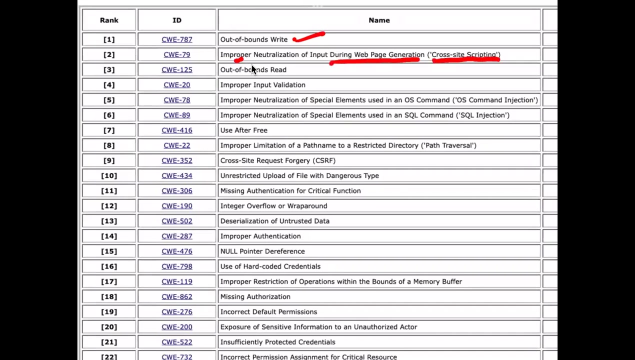 okay, let's expand. okay. so the rank number one is out of bond, right? something that we just studied, right, okay? and then second: uh, heavily used weakness by hackers- of course cyber criminals- is improper. neutralization of input during web page generation is called cross-cutting site scripting. we'll study that. then there is something called out of bound, right read. 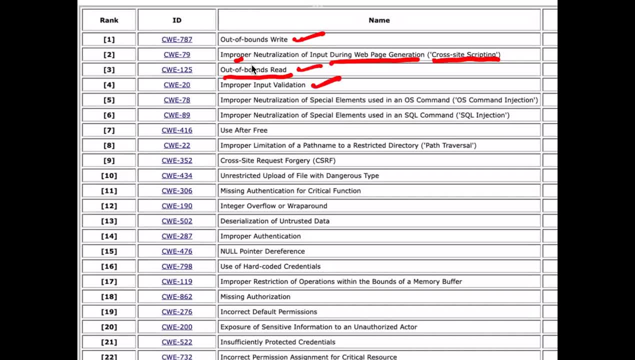 earlier it was right now read: improper input, validation okay, and so on. you can go through the list. integer overflow is another overflow. we have studied in computer architecture course what is the overflow and how. integer overflow can give malicious results, right, wrong results, and this can also be exploited. null pointer dereference: this is another issue, right, many programmers 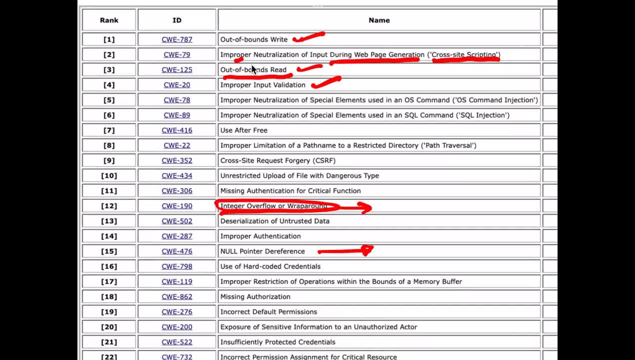 don't know how to use pointers, how to, you know, initialize it and so on, then hand-coded credentials- it's kind of backdoor in my understanding. right, i mean hand-coded credentials. is that you know? i mean the code. you say that if user is x, then allow and then x could be your name. right, if you're a developer and you create a code that, 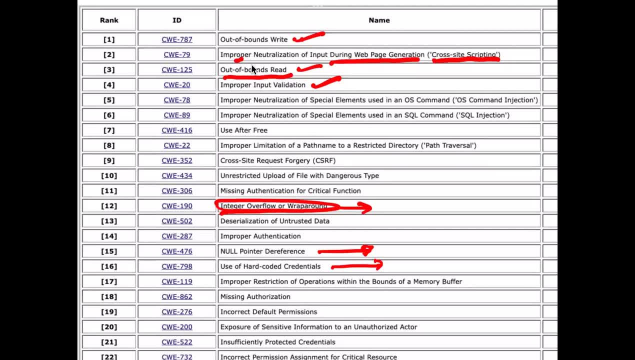 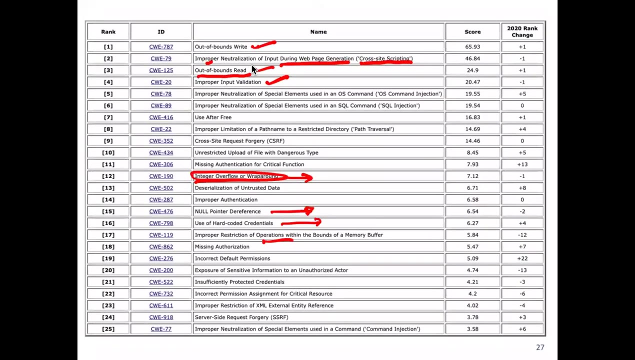 if user process id or user id or owner of process is, say, your name, then allow following x's right. so this hard code can be very dangerous because you think nobody will know this, but cyber criminals are smart enough to find such gaps out. okay, missing authorization. incorrect default permissions. 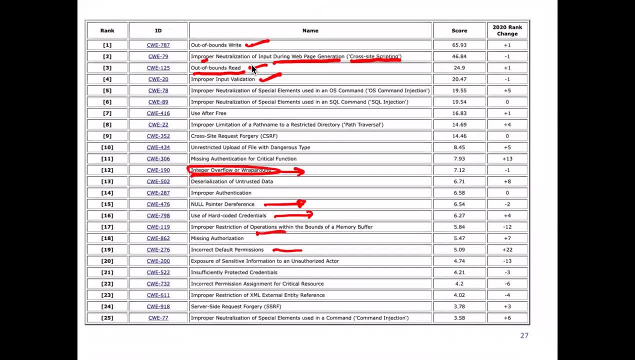 and so on. okay, please go through this list, and this list keeps changing. but something that is interesting is that something that we are studying now is heavily exploited at vulnerable. this is still ranked one and this is known to everyone, even window, the one you know. microsoft knows that this is their vulnerability, linux knows this one, intel knows this is the one. 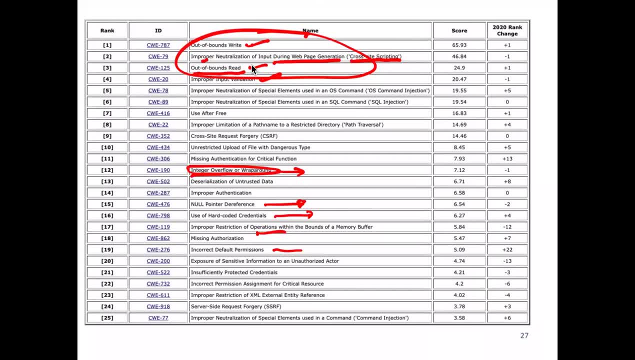 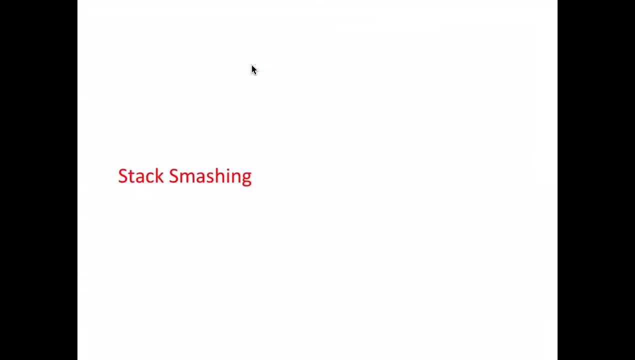 the ability and they have also designed solution for that. but this again, the solutions are not hundred percent full proof. okay, all right. and there are old servers with where you know, with with old os and so on, or old chipset where this vulnerability still exists. okay, so let's come to more interesting part called stack smashing. so so far we have seen: 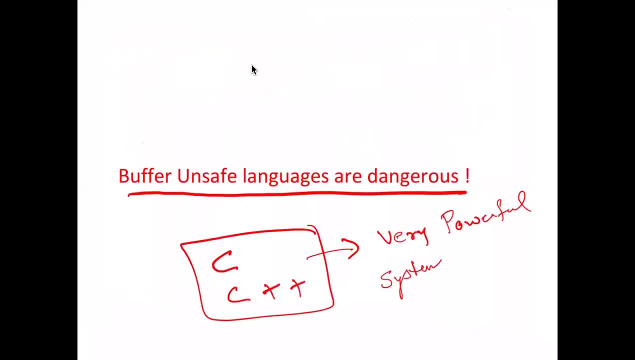 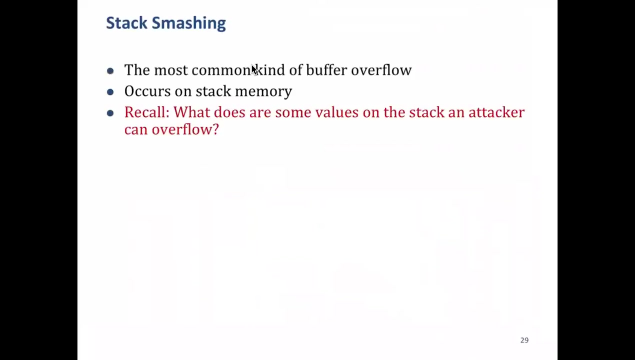 that by overwriting we can create some problem in the system. right, okay, but still we have not discussed how we can take control of the system. okay, so now let's look at stack smashing again. this comes from the same paper which we referred in the beginning. all right, so this is most common. 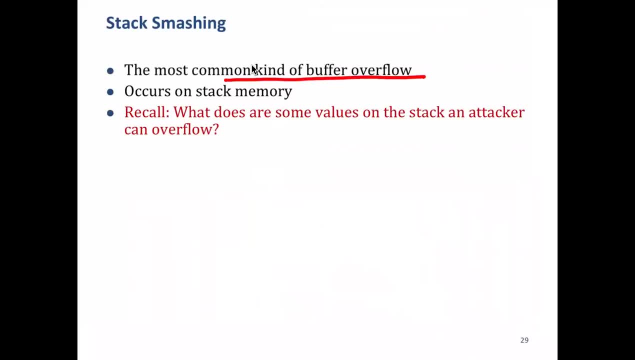 kind of buffer flow problem it is occurs in stack memory. that's the word stack we use. okay, so so now we have studied stack in the last class. that's the reason we spent one full hour to understand the concept. so what are the values in the stack that an attacker can? 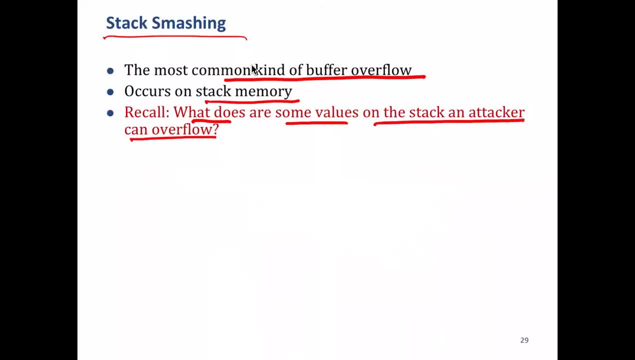 overflow and attacker will like. attacker may not just want to, you know, crash your system it may, but you know that's not really a smart thing. right, crashing a system is pretty simple for a hacker, okay, but but more than that, taking control of system is bigger, you know, challenge. so what is the value? 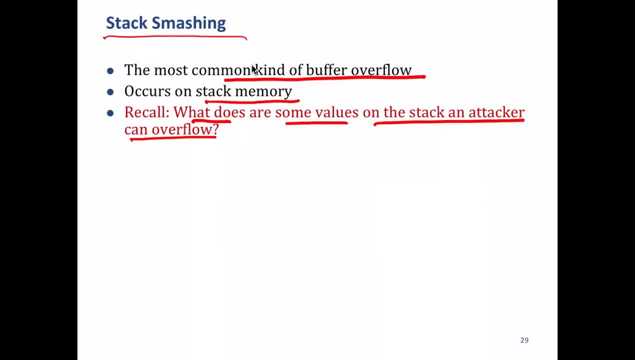 that you studied is most exploited. yesterday we discussed this. anyone changing program point? yeah, so basically, what we save in stack is variables. okay, various variables. come then we have arrays, we have a stack. okay then, apart from that, two important things is that when we make a function call: 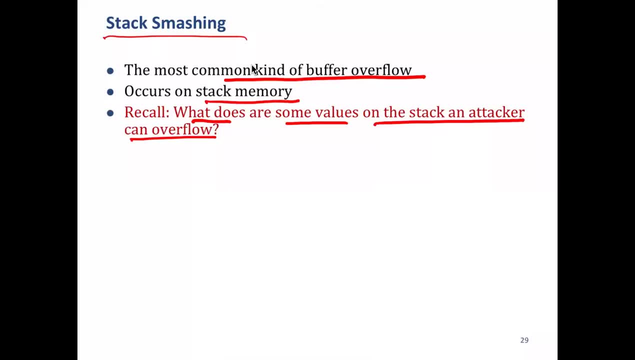 then we store previous functions, which has our caller functions. two things right. first is the starting, where starting frame, starting address okay and where it should program count. you know when, when the new function, there's an execution, when it's complete, where the control should go back okay. or the program counter, which we call it, is a section pointer in. 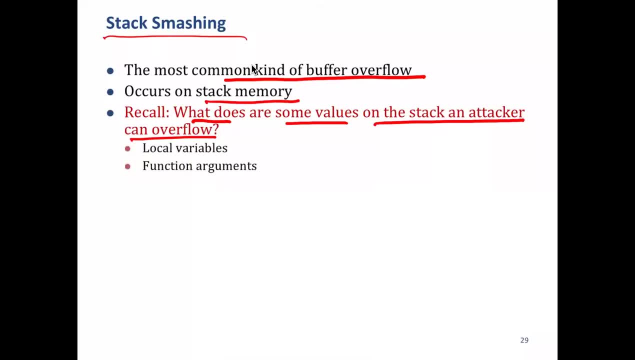 intel terminology. right, so these are. so these are the things we save: local variables, function arguments then, where the frame of the caller function is starting, so this is a caller function, okay, and- and this is note that this is also in this stack right, and so the so there is a stack frame. 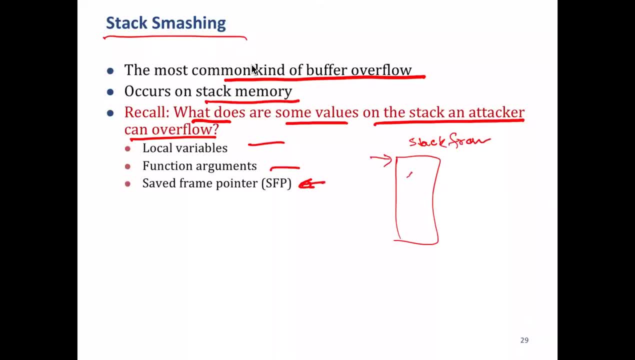 so now, when this caller function in the color function, starting address of the frame is given by frame pointer and then stack is at the top. stack pointer- oh sorry, stack pointer- is at the top, and apart from that in the text segment there is a counter called program counter, or we call it instruction pointer. 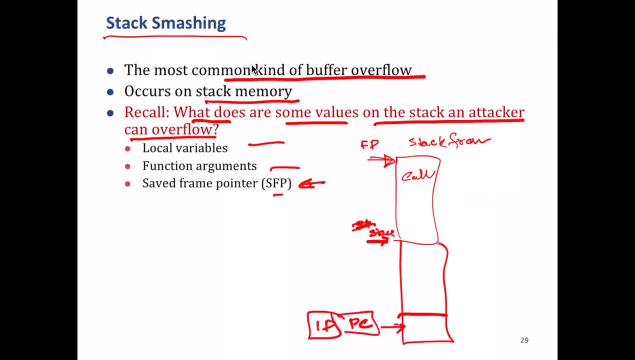 in intel. both are same and we'll say which instruction we are going to execute next. okay, so now something. that's so when, when this calls a function, then another stack frame is created, let's say it's created here, uh, okay. and when the execution of this is over, then again. 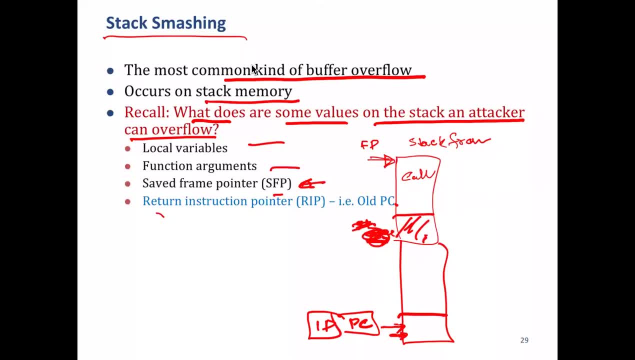 next instruction will be executed. you know from where it stopped, so something that's really really important is program pointer or instruction pointer of caller function, which was saved in the stack. now, if we can overwrite this right to different address, then next instruction that will be executed after the call function is over will be something that hacker wants. 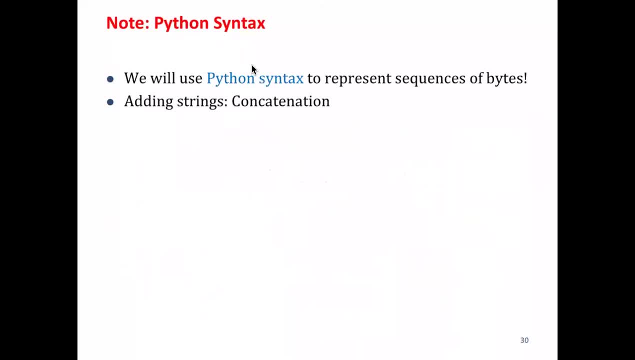 okay, so now you know before that, um, we'll use little bit of python syntax to illustrate our concepts, so don't worry about, we are not going to compile it, and so on. but you know this right, some of this right, when this, the abc plus def, becomes bigger string called abcdef, and then when a is multiplied. 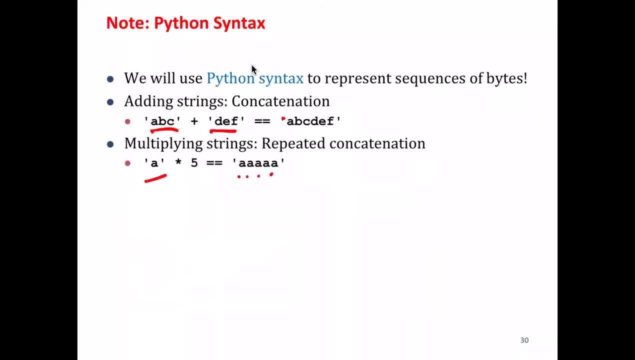 a star five becomes five times a in this string, this concatenation and so on. so there are many things you would have studied. so we'll use some of these- not much, but you know, just just for you, because once you get this audition, you shouldn't get confused. okay, so let's look at this. 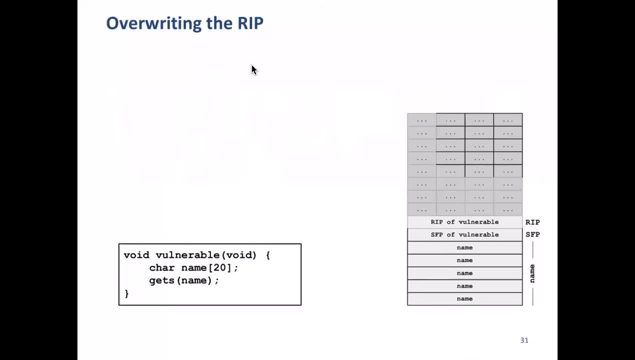 this code: okay, this is c code. okay, char name 20 and then just gets name. so this is for name, up to this and before that you will see that instruction pointer, old program counter on instruction pointer is stored. that's of the caller. the caller is calling this right. 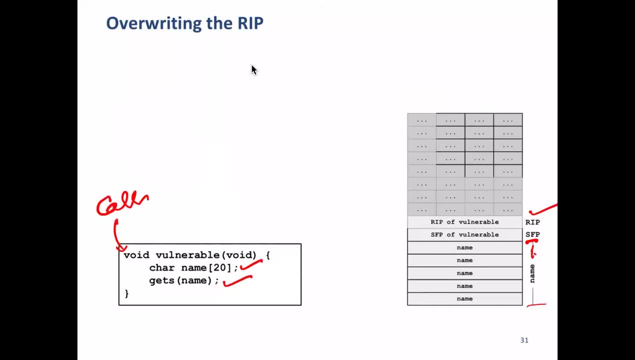 caller is calling this, so. so once the instruction pointer is stored, execution of this over. it will go to caller next instruction. so all right, and so it's like this. okay, so get will start writing from here. okay, and now attacker wants to execute. instruction of address: dead beef. okay, so basically there is some some address dead, dead beef. okay, let's assume it's here. 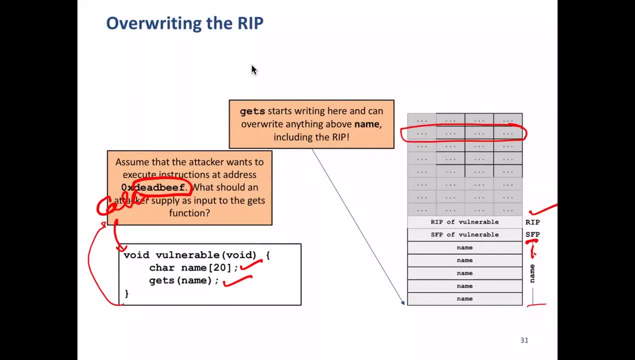 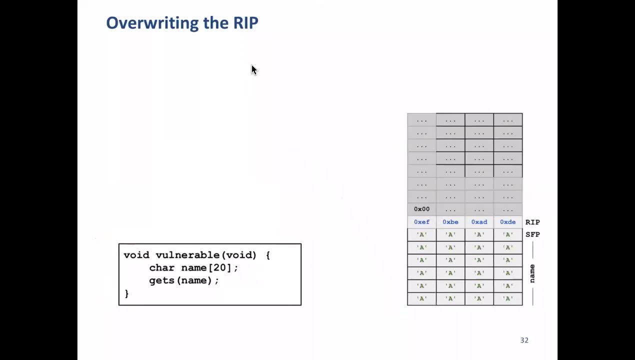 or somewhere- okay, and then it wants to execute that. so what we'll do, it will start putting values here and put dead beef here- okay. so it's like this: it will put all whatever junk characters like a- okay, and then spf also, it puts a- okay, and then here it puts dead beef. if you, if you want to put dead beef here. 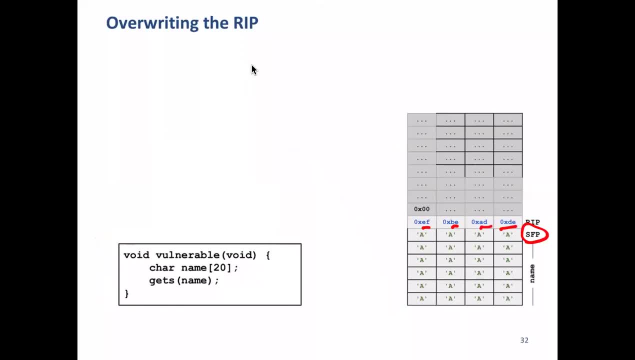 so you can see this is a little ndn, so you can see d, e, a, d, b, e, e, f here, right, and then termination. this is for termination, because you know it's like what? what do you call the new line character or whatever? okay, so now. so the input is this one and it is over, written over both, you know, written in. 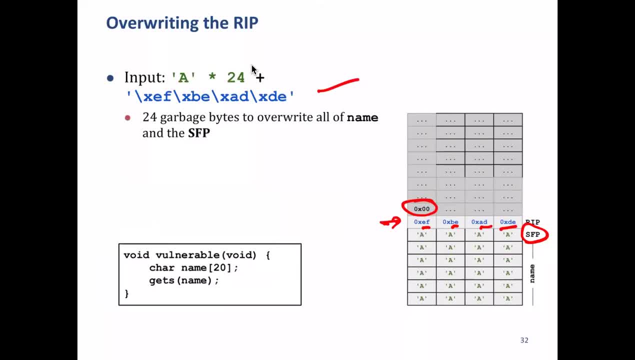 section pointer: written or saved program counter, and then, uh, frame pointer: okay, and when execution of this is over, control goes back. okay, then uh, basically the old program counter is popped out and next instruction to be executed is something that's that's in the program, popped out program counter. 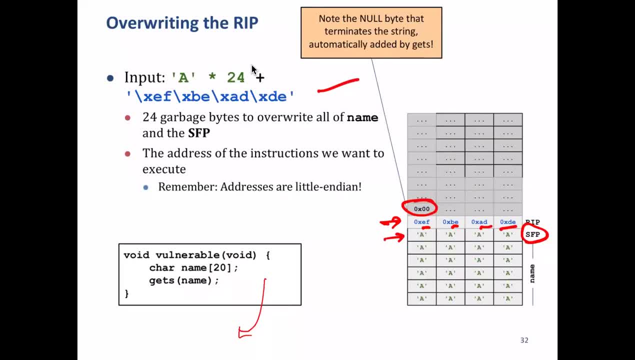 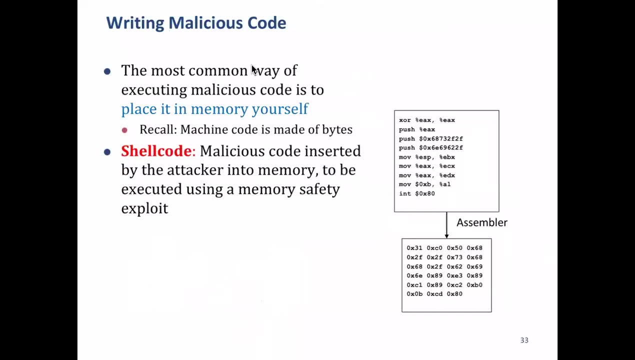 okay, all right. so this way, you know, this way, uh, code can, uh, you know, uh, malicious code can execute. all right, all right now. the most common way of executing malicious code is to place the code in memory itself. okay, now we have said that we are jumping into certain location now, and that location, that malicious code has to be there. but 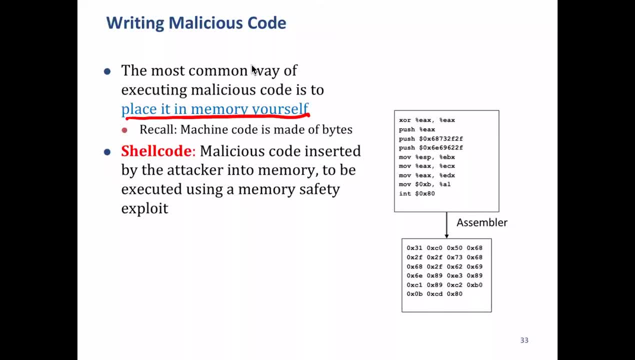 how does code go there? okay, this thing is it's not working in this way. we have to think, and that sort of thing for aальную um, but uh, so we'll have to think that how you are unwell. you got to think that how you are going to place the malicious code. also, right now, we 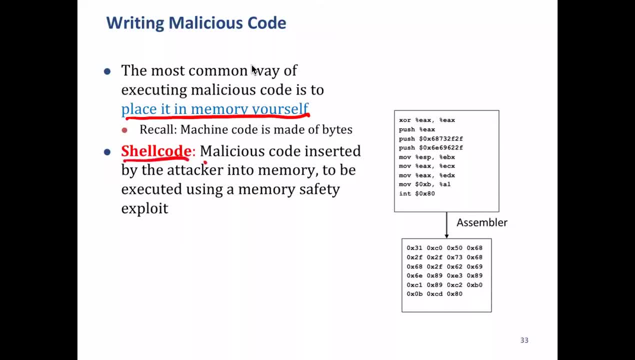 have manipulated only jumping address or malicious code. okay, so there is something called shell code. okay, it's malicious code is inserted by the attacker into memory to be executed using memory's safety exploit. okay, it's called shell code because usually spawns uh, a shell or terminal. so we'll look at how. 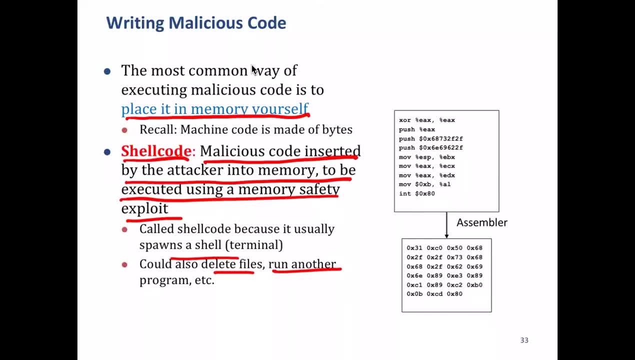 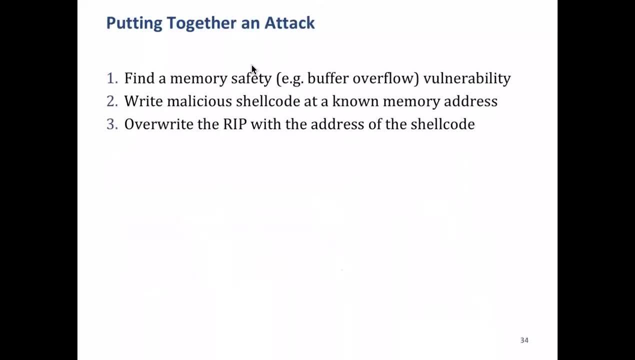 file and it can encrypt and do a lot of other things. okay, of course you know whatever shell normally can do. okay, it's all right. so now, uh, attack is as follows: find the memory safety vulnerability. there's a first thing that attacker has to find out: is there a vulnerability of this? 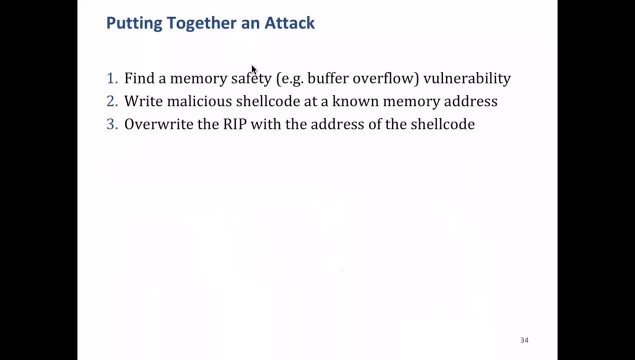 kind, okay, uh, there it. and for that, you know, attacker may experiment for months together and so on, or use some tools which will generate certain sequence and of input and try to crash the system and so on. and you know it's like a role of a doctor right looking at patient. 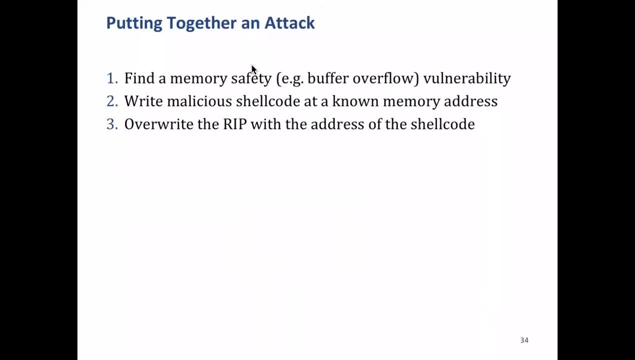 this has to find out that something is wrong. is there something wrong or not? similarly, here, attacker has to find out: is there something wrong? so first thing he's going to find out: memory was safety vulnerability. click buffer, overflow okay and then write malicious shellcode and known memory address. 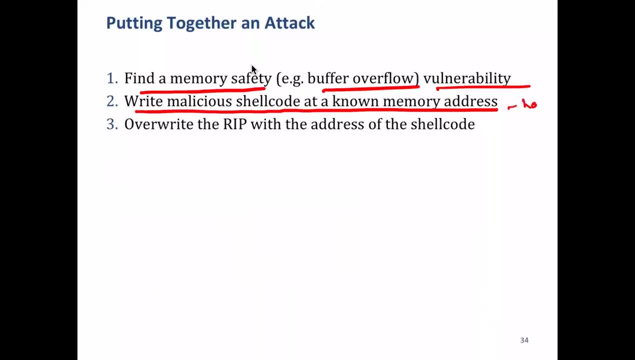 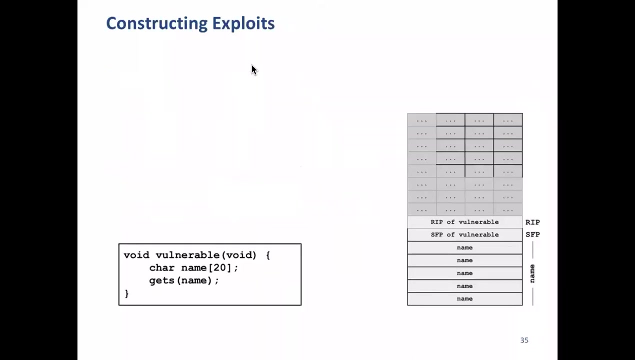 fine how that you can find out. okay, do little bit of googling so we'll tell you one way. okay, overwrite the review, the address of shellcode. okay, now return. then return from the function. then obviously return goes to malicious shellcode. that's it right. so let's look at this example. 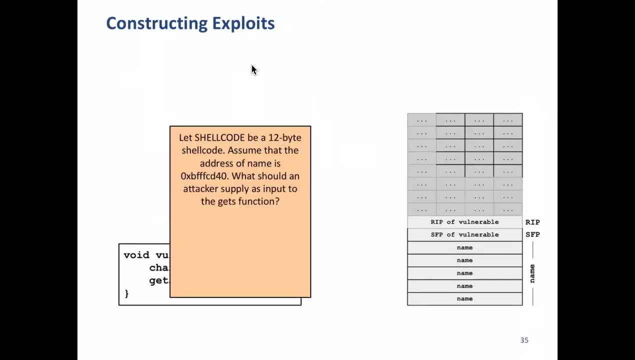 so this is the code. so shellcode is, let's assume so this is the code which is correspondingly stack is here, and then shellcode is, say, 12 bytes long. okay, and assume that the address of the name is. okay, the address starts from here. okay, so now what should be the input? 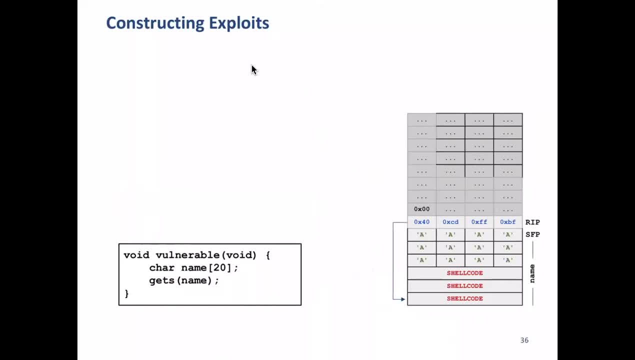 okay, so let's look at this, so let's see what we can do here. okay, so let's say, shellcode is a 12 bytes long and the shellcode is a 12 bytes long, so we put this on right, okay, so now, uh, you put shellcode here. 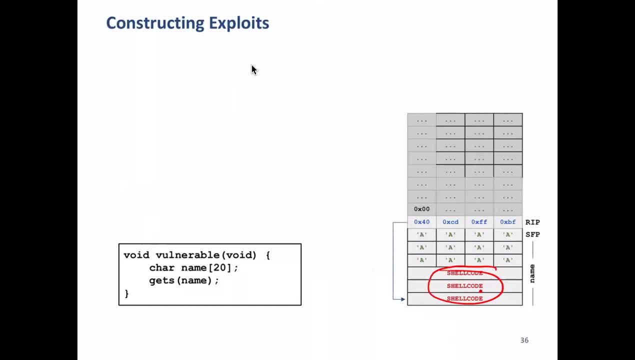 so instead of putting all a, since it's a 12 bytes, so you put shell code here and now- uh, you know this rip- you should give address of where the shellcode is starting now. so when this program gets over and you give this intelligent input of all these aas and return. 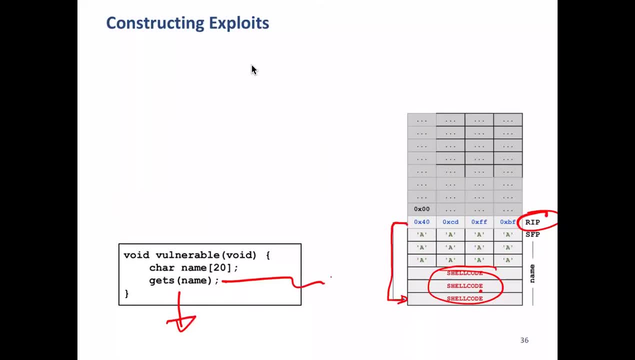 address and when this gets over, new old pc is loaded, and then old pc is nothing but this point and then shellcode. as a result of that, next instruction to be executed corresponds to first section of shellcode. okay, so this should be your input. all right, okay, so alternative is that you can put shellcode here. 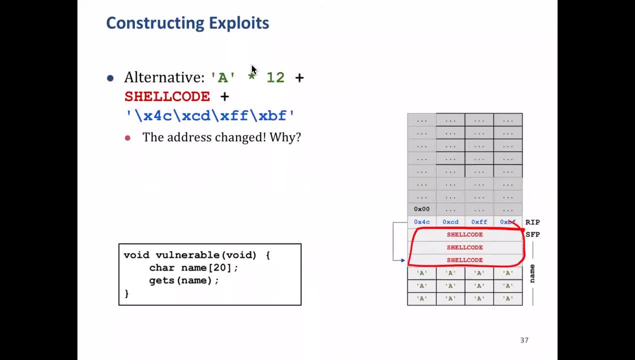 okay, and then accordingly you'll have to give the input, so it should be 12 times a, which is here, then shellcode and then return address. okay, now the question that comes so here, after it returns- it will come here because return pc is- will point to this instruction. 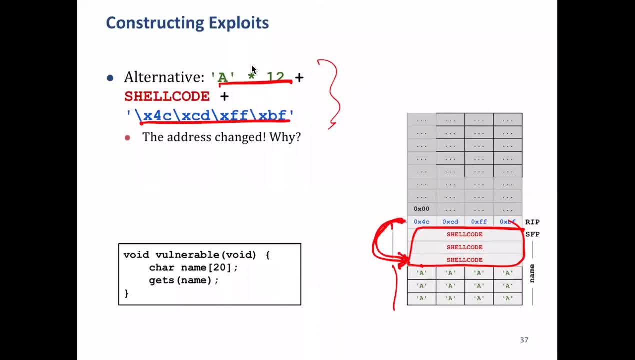 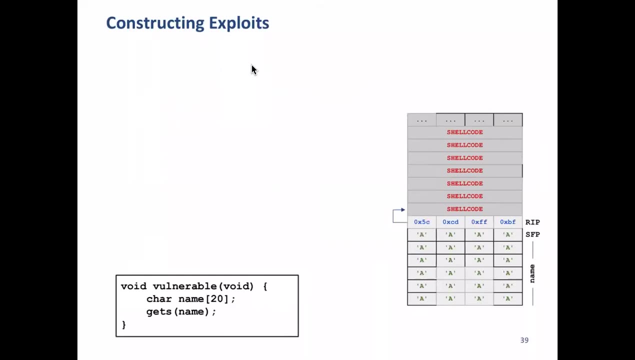 what the question comes to your mind. if shellcode is more than 12 bytes, then what to do? then? you can put shellcode here anywhere in this side. okay, so you can put shellcode here and put intelligently all these characters and then put return address as a beginning of where shellcode starts. this one: 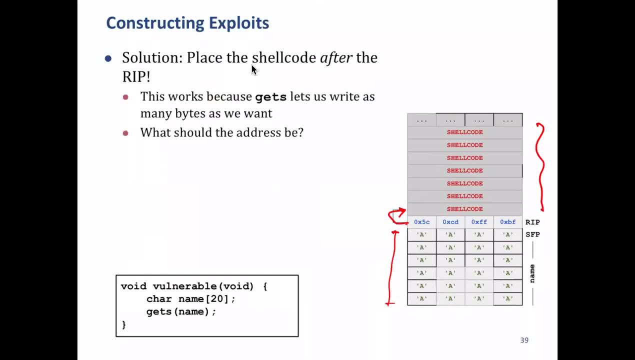 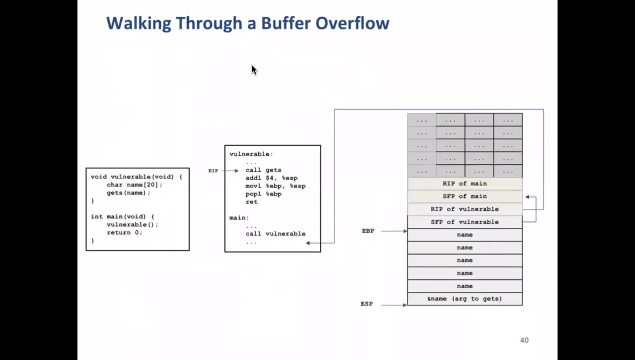 all right, okay, any question? no, please go to ppt, you will understand it, right. okay, so this you can walk through. this you know, because now what we have been doing is we are looking at only in terms of c code right. c code is not known, so we are looking at only in terms of c code, right. 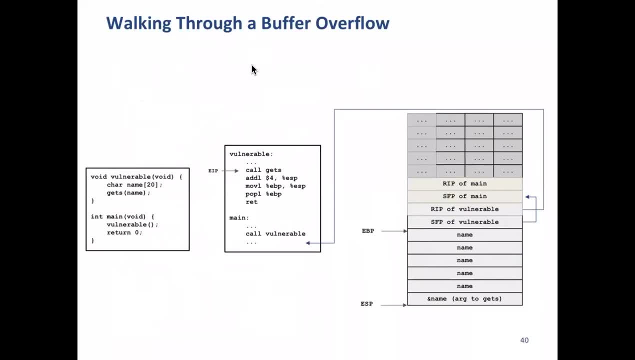 so if we were to run new learned by likeness we would have to look right satisfactorily. so lets assume the native is the same. as you have always used a link to attack a right, so let's assume that how does it run from corresponding machine instruction? 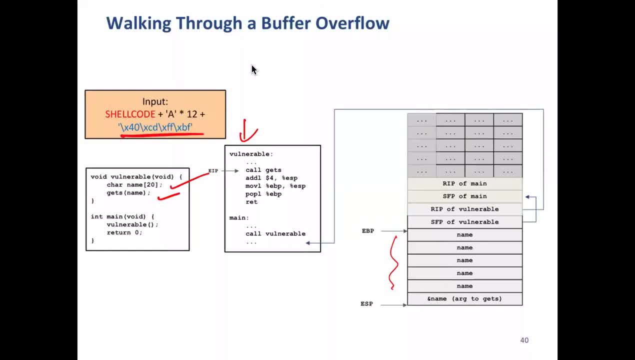 now, of course, is assembly here right same thing you can see here: shell code will come here and then a. so first shell code and then a. okay, uh, so now 3, 12 a's will come, so this a's will get over. return over. okay, just a minute. 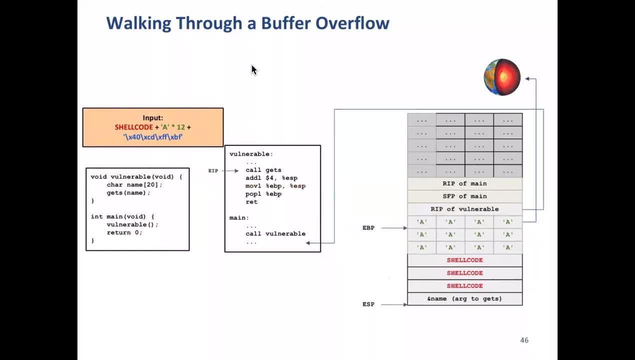 okay, so a also gets written over starting frame address. so now that is also becoming corrupted. now, once you write something here it will point to some area, something, some junk, okay, so anyway, the program execution is uh and you know, will get disturbed and then rip of unrable. 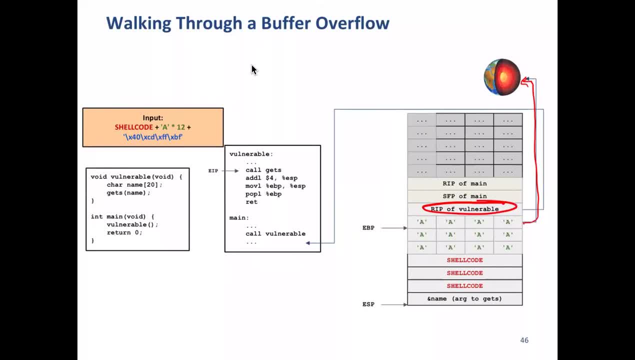 you know will get disturbed and then rip of unrable. you know will get disturbed and then rip of unrable. you will have to write to which which was pointing to next instruction in the code. now it will point to this one beginning of shell code: okay, and accordingly, you know, your stack pointer etc will change. 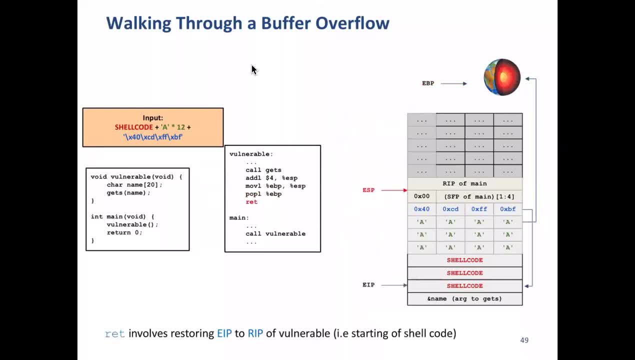 all right. so here is shown, i say, how stack pointer and eip will change when this execution happens, where you now you can see in the red where the current instruction is being executed right, okay, so you will see that how different both stack pointer and e base pointer uh will change. right, and we have seen study this in detail. 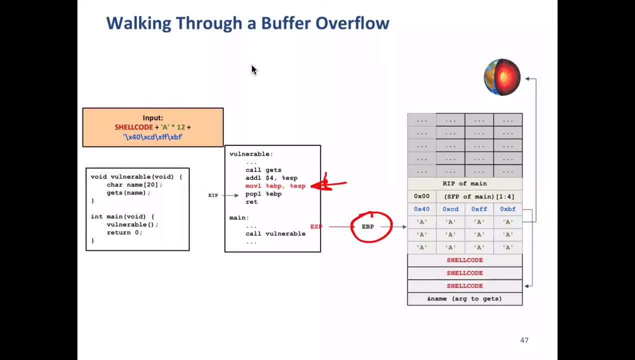 in the last class. so you can now make out all right, another two minutes and we'll close all right. so this is quite simple. you can see that. let me just okay. when instruction just a minute after this. when this is executed, then it will start filling shell code, because input is this one. 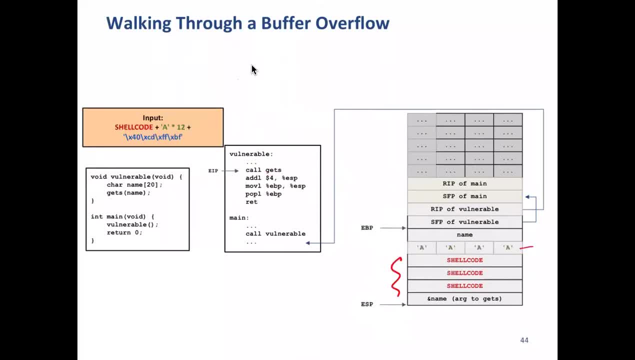 okay, and as a result of get again, the 12 times a will be written here. so now we can see that spf gets screwed up. okay, and then we write appropriate value of rip, return instruction pointer or old pc which will now should point to the this starting: 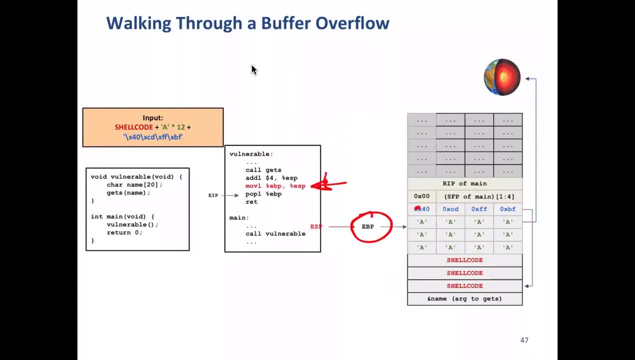 address of shell code, the one here, right, okay, shown here, all right. and when you know when this execution is over, it comes to return. return means that now you load the old program counter and then, as a result of that, yeah, so okay, as a result of that, this rip. 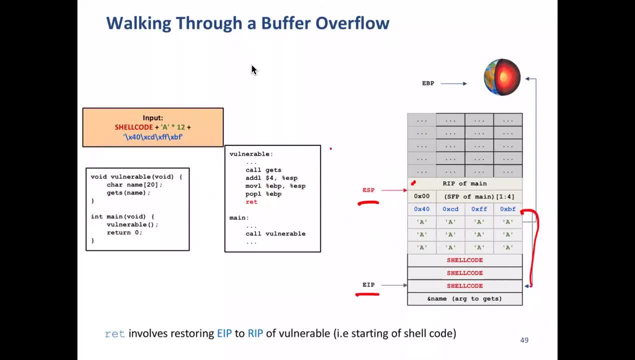 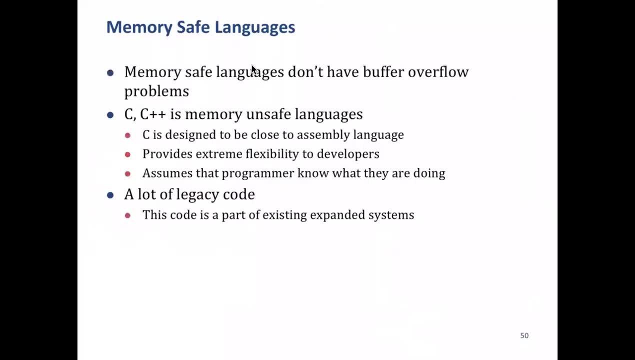 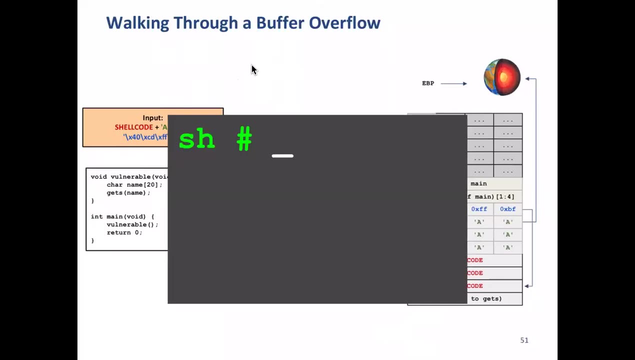 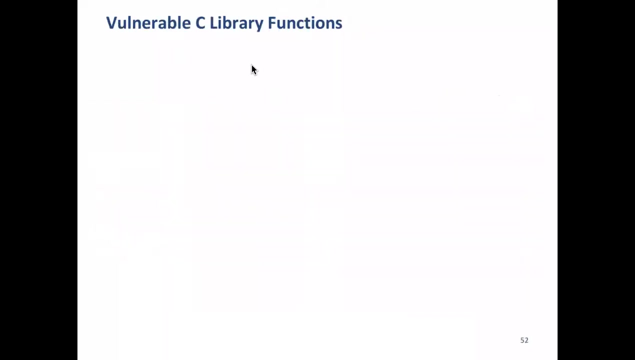 okay, sorry, this return instruction pointer will point to the beginning of the shell code. so that's it all right. okay, and when this executes, then if the shell code is appropriate, they will get shell and then you can exploit things, okay, any question, sir, i have a question. yeah, yeah, so everything in the staff frame, it is uh. 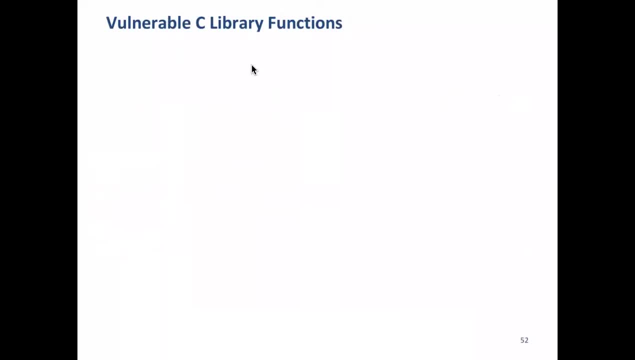 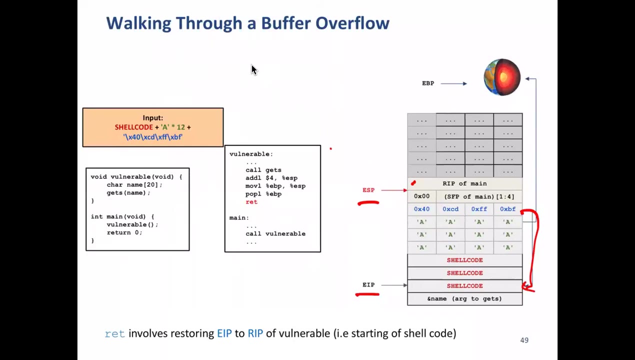 like initialized in runtime, like this design, and how will the hacker know that he have to place this address like: can you go to the previous slide? yeah, yeah, yeah, yeah, yeah. so here, like we know that there are these many bytes after shell code which we need to fill. 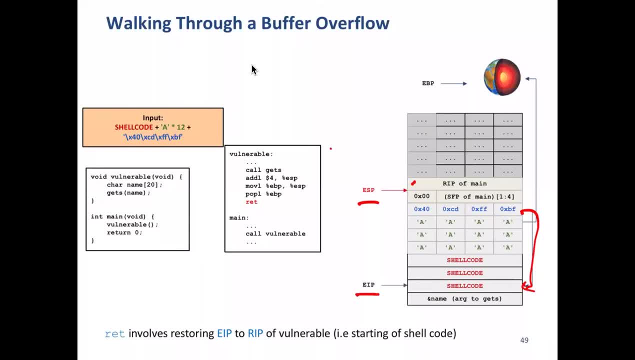 with a, a and then we know the address of the. what address we have to fill. we have to basically fill the shell code address, but everything is happening at runtime. then how will the hacker know that this much amount of space is left and he have to write, overwrite here this address and all that? so? 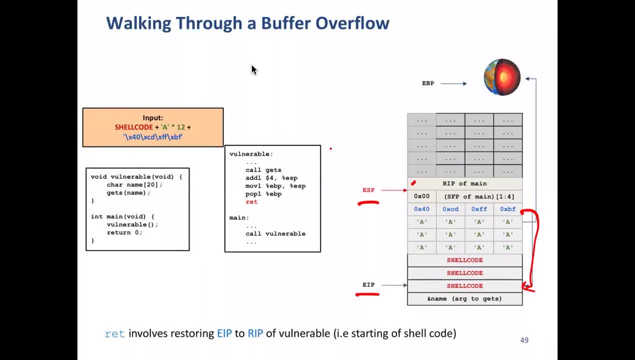 a lot of stack designs are known, okay, so it's not that totally unknown things, right. i mean, for intel and other processor is kind of published, it's, it's known, and then, uh, there are, of course, there are. you know, when a stack is created then it has to reserve some areas, right, okay. but all this is 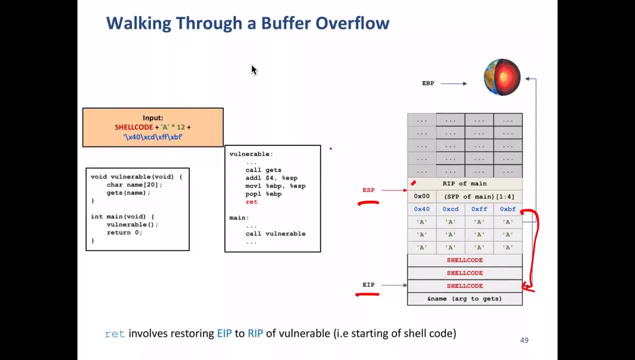 based on experimentation. it's not that you know, once you know that there's a, you as a hacker, know there is a vulnerability. you can just write something and and then it works right. so it's based on experimentation. you know, basically, how do, how do you know? this is a starting. 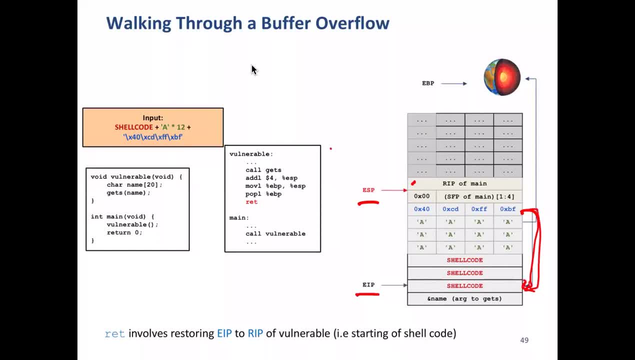 address and even that addressing is after every execution, like one time, uh, when we use, when we execute the address, my yeah, so uh, for the next time, yeah, but uh, yeah, so all these things can have to be see. all these are relative address somewhere or other, right? 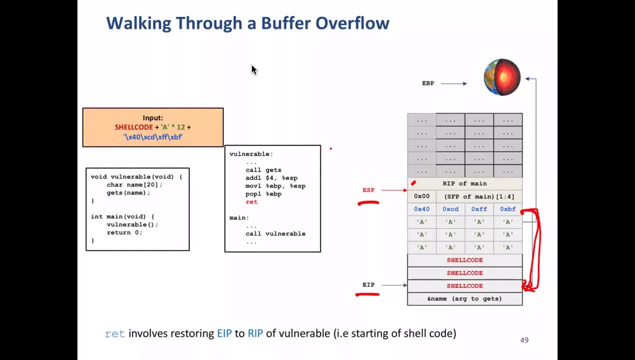 Yes, sir. Okay, you know. I mean, the way stack is actually filled is also relative to base pointer somewhere, right? So all these things are you know. hacker will of course know what is size of shellcode, okay, And it will know relatively relative position where it. 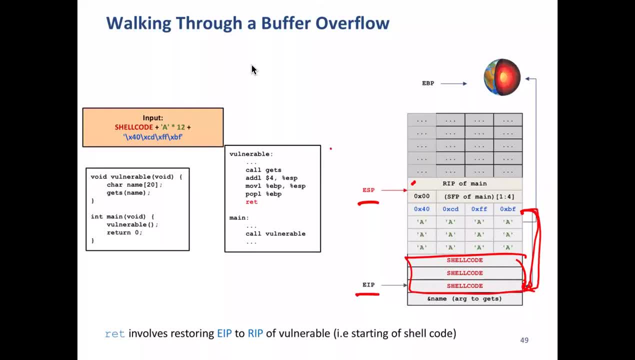 has placed the shellcode. Okay, based on that is all, experimentally, he or she has to do to find out what is the address, right? Yeah, you're right. So it does not come by, just you know, looking at it and so on. That's the reason: hacking is not that simple, Okay. 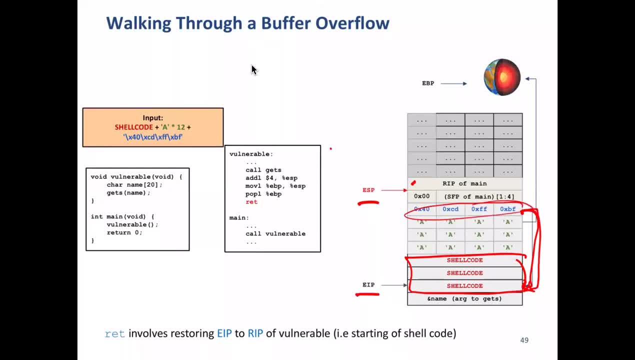 so this value you can write junk. that's very simple, But accurate value is comes through. you know some wild guesses and then some previous experience and so on, so forth. right, And some other information that you have about where exactly. 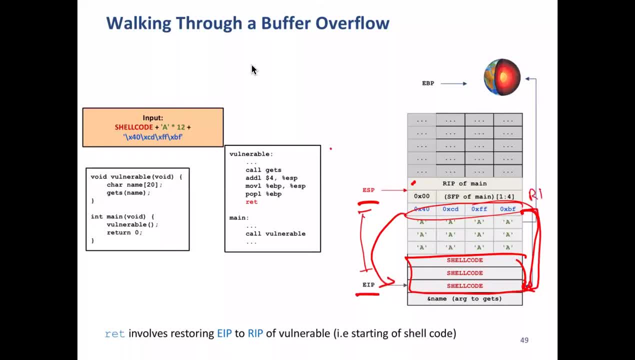 in relationship to this data, our IP, where should it be, and so on. It may require 100, maybe 1000 attempts, and so on. Okay, Yeah, Okay, Yeah, Yeah, You can experiment. this actually will give a exercise and then try experimenting with. 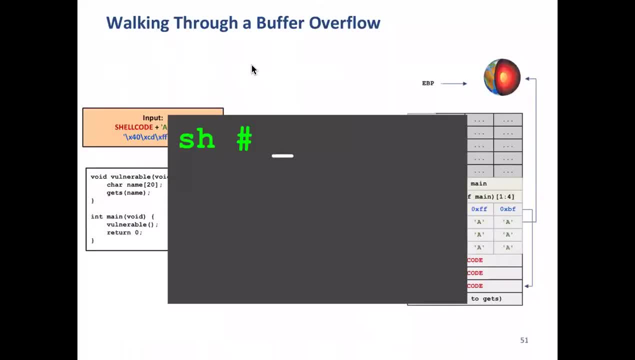 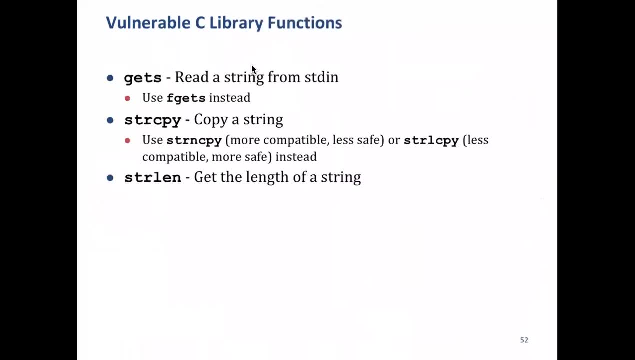 it All right, Okay, so that's it for today. So we have vulnerable C library function gets, and there is solution for that. there can be. you can use F gets instead of a string copy. you can get STR and CPY Instead of STR and LAN, you can use STR and LAN. Okay, all these.